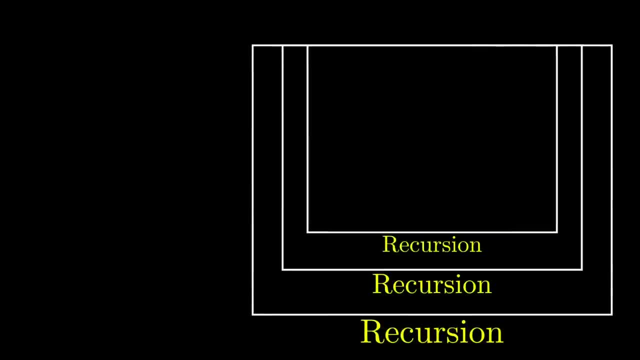 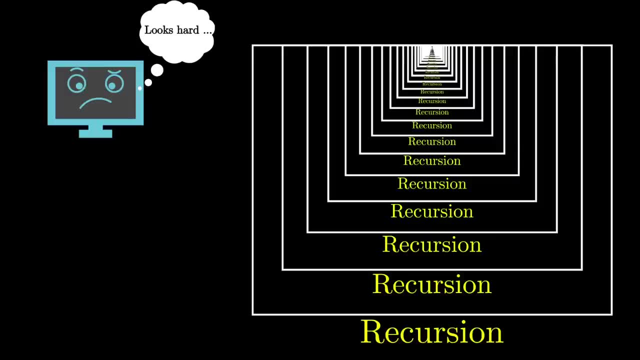 Today we are going to talk about recursion. I think most computer science students would agree that recursion felt more confusing than your average computer science topic. In this video, I'm going to show you five simple steps that you can use to help you tackle any recursive problem. 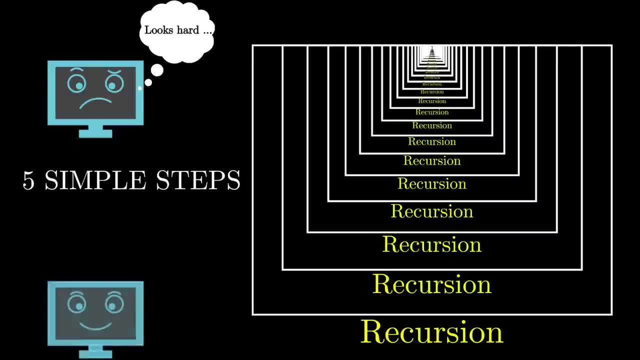 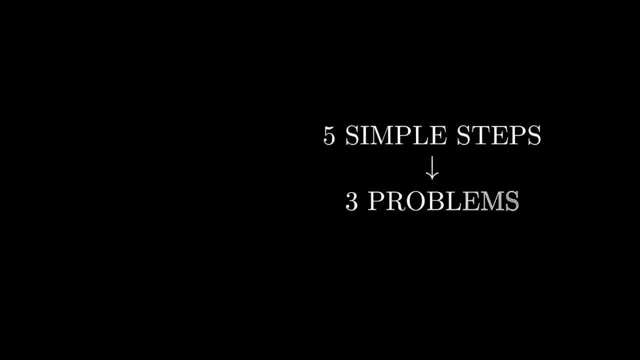 and hopefully these steps will help you realize that, in reality, recursion isn't actually that bad. I'm going to show you how to apply these steps in the context of solving three specific recursive problems, each of them progressively more difficult than the last. so make sure you stick. 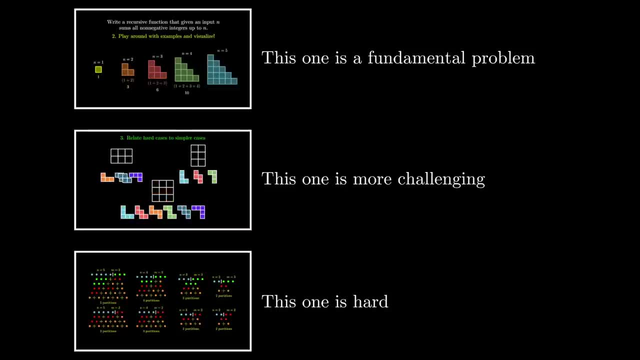 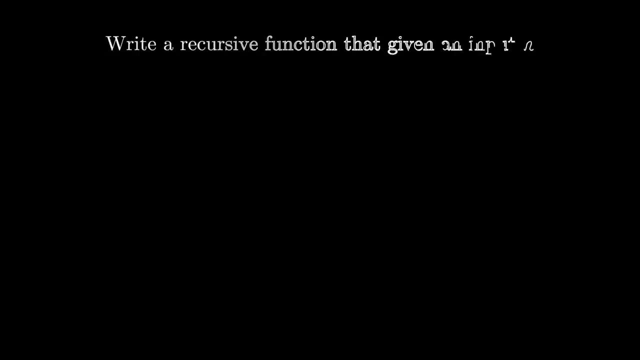 to the end of the video And, as always, I think you'll get the most out of this video if you take the time to pause and ponder some of the problems that we worked through and the steps we went through to solve them. So, without further ado, let's get started. Suppose we want to solve the 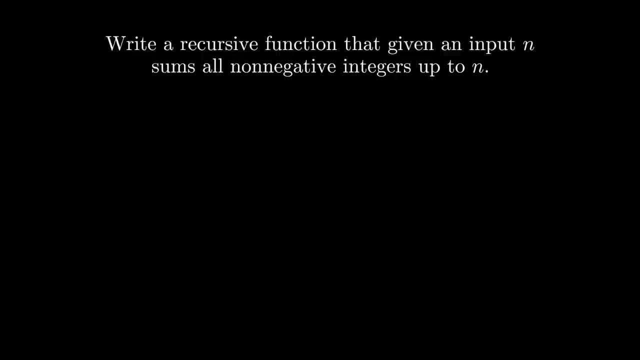 following problem recursively: Write a function that, given an input n, sums all the non-negative integers of the following problem recursively. Suppose we want to solve the following problem recursively: Write a function that, given an input n, sums all the non-negative integers of the following problem recursively: Write a function that, given an input n, sums all the non-negative integers: 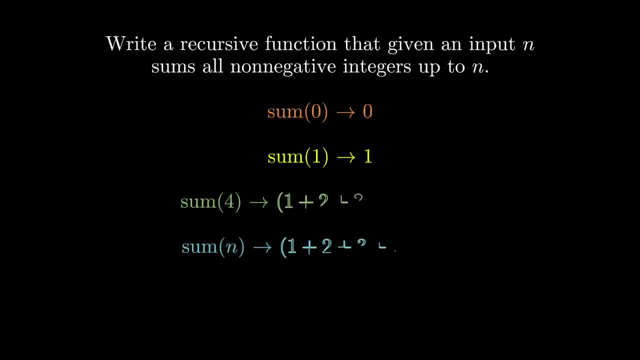 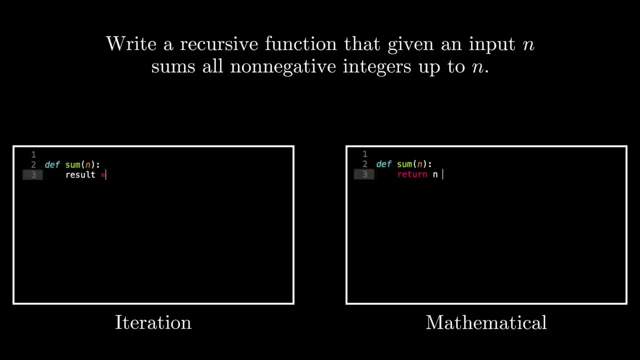 of the following problem: hist input. Here's a couple quick examples of inputs to this function. Here's a couple quick examples of inputs to this function to give you a sense of what A lot of you may have seen an iterative version of this function or even a mathematical version. 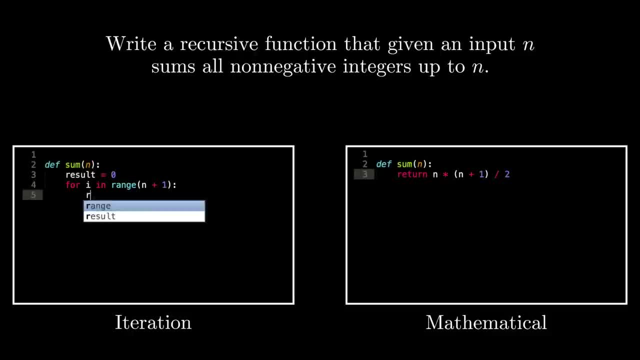 of it that we went through in a previous video. But if you had to solve it recursively, how would you do it? Recursion is all about taking a problem and solving it using simpler versions of the problem. so the first step in solving a recursive problem requires you to. 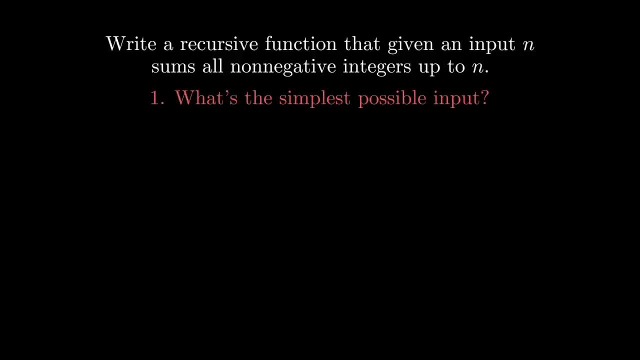 to ask yourself what's the simplest possible input for the function. Here the simplest possible case is n equals zero, where we know that the result should also be zero. The simplest case often translates itself into a base case for our recursive problem. The base case of a recursive function is the only input where we provide an explicit answer. 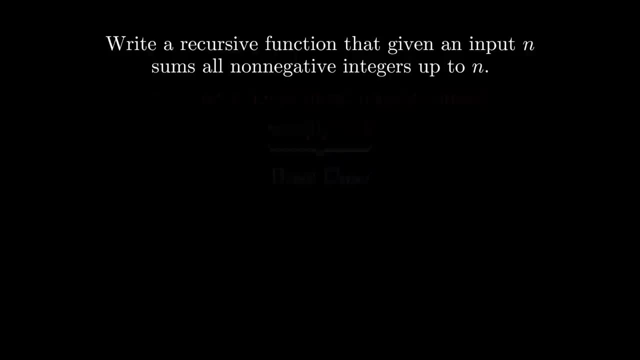 All other solutions to the problem will build on the base case. The second key step to solving recursive problems is trying examples and visualizing how the inputs and outputs of these functions interact In this problem. one fun way to visualize things is to treat our sum as building a triangle. 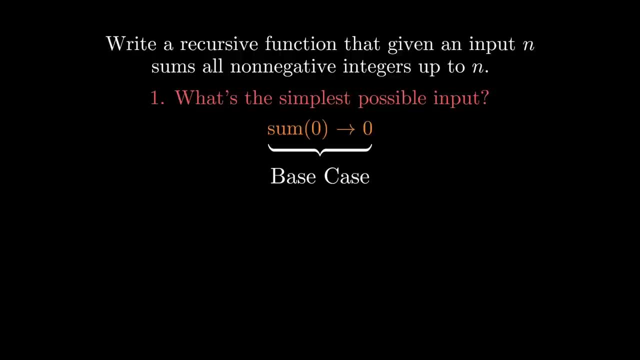 The base case of a recursive function is the only input where we provide an explicit answer. All other solutions to the problem will build on the base case. The second key step to solving recursive problems is trying examples and visualizing how the inputs and outputs of these functions interact. 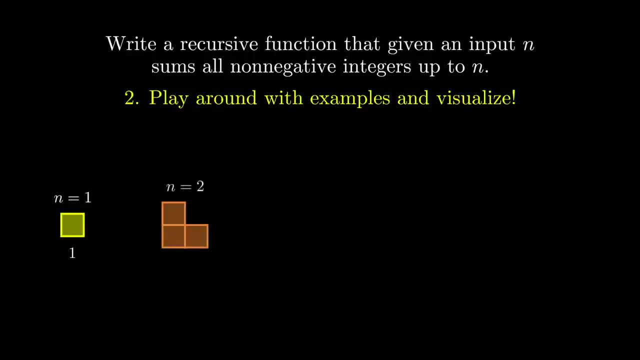 In this problem. one fun way to visualize things is to treat our sum as building a triangle, with the base as the input value. That way, our sum is the total number of individual blocks in this triangle. You can try as many examples as you want. 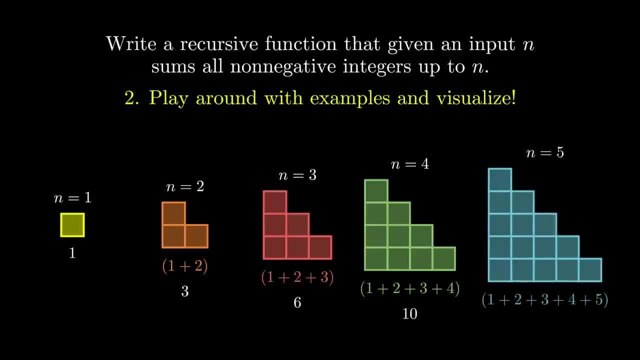 Once we have a set of examples, we now want to move to the third step, Which involves relating larger examples to smaller examples. Take a second to see if you see any relationships between the cases here that pop out to you, Put in more specific terms, with these examples. 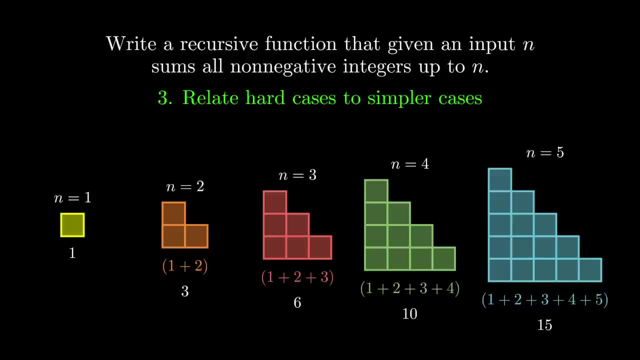 Ask yourself: hey, if I was given the answer for the n equals 4 case, could I solve the n equals 5 case? If I was given the answers to the n equals 3 case, could I solve the n equals 4 case? One interesting relationship that you may have noticed. 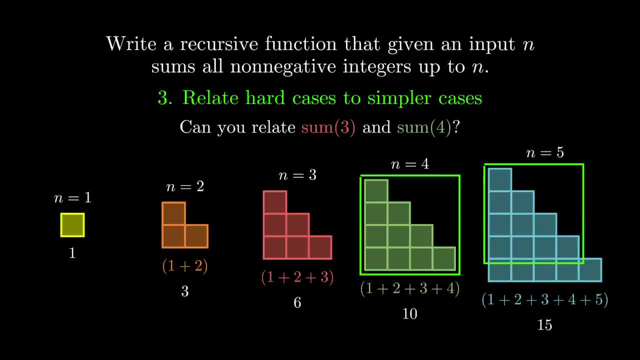 is that if we know the answer to the n equals 4 case, all we need to do is add 5 to this answer to get the solution to our n equals 5 case. And similarly, if we know the answer to the n equals 3 case. 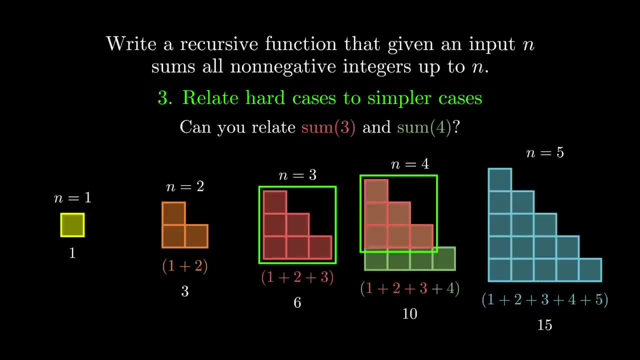 we can get the answer to the n equals 4 case by adding 4.. And it's not too hard to convince yourself that this should be true in general. But, if necessary, feel free to try some larger cases to verify. This now brings us to the fourth step. 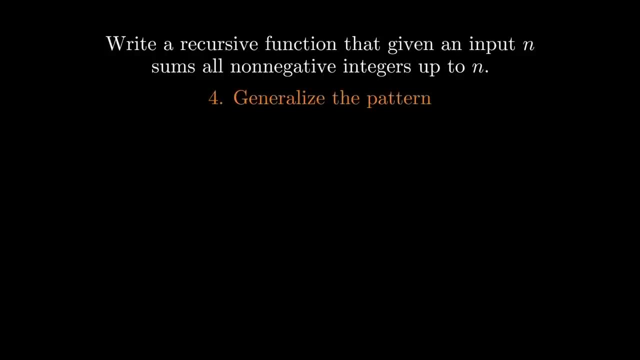 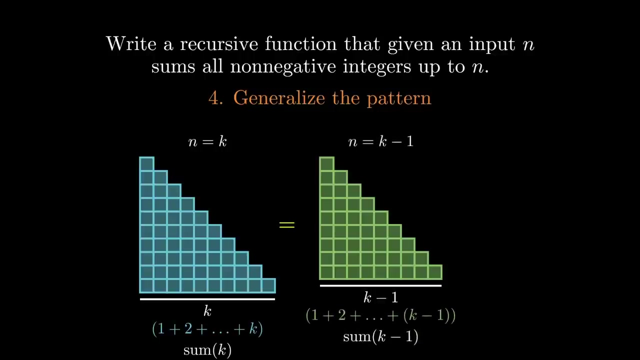 Key step, which is to generalize this pattern. Let's say we want to figure out the sum for the input: n equals k. We can find the sum by first taking the sum up to n equals k minus 1.. And then all we have to do is add k to this value. 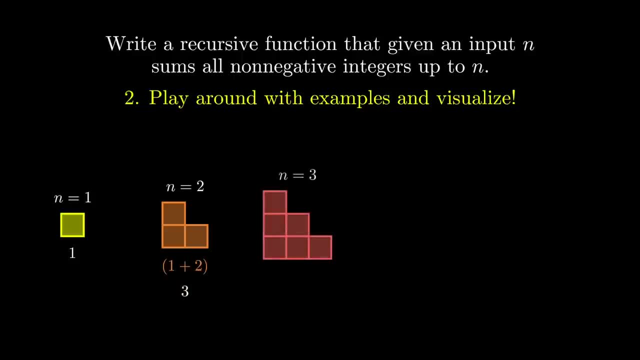 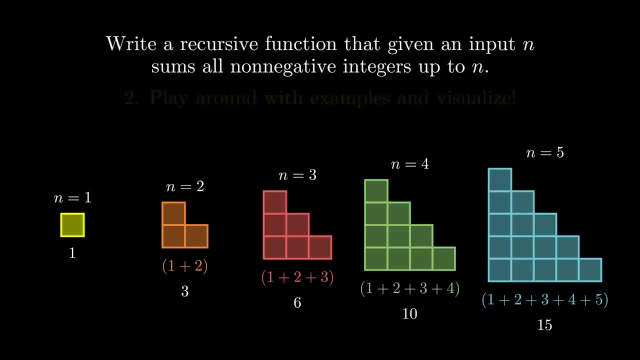 with the base as the input value. That way, our sum is the total number of individual blocks in this triangle. You can try as many examples as you want. Once we have a set of examples, we now want to move to the third step, Which involves relating larger examples to smaller examples. 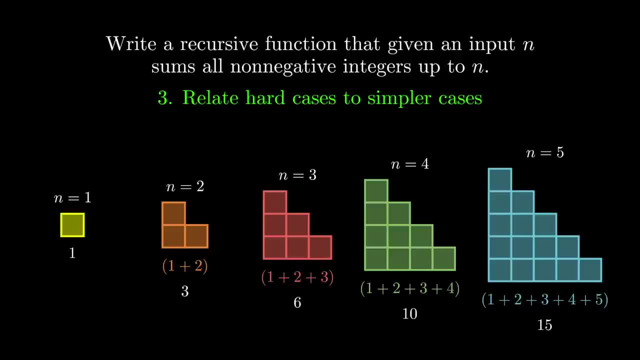 Take a second to see if you see any relationships between the cases here that pop out to you. Put in more specific terms with these examples, Ask yourself: hey, if I was given the answer for the n equals 4 case, could I solve the n equals 5 case? 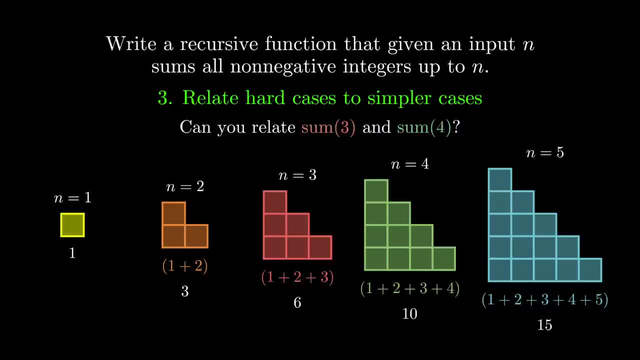 If I was given the answers to the n equals 3 case, could I solve the n equals 4 case? One interesting relationship that you may have noticed is that if we know the answer to the n equals 4 case, all we need to do is add 5 to this answer to get the solution to our n equals 5 case. 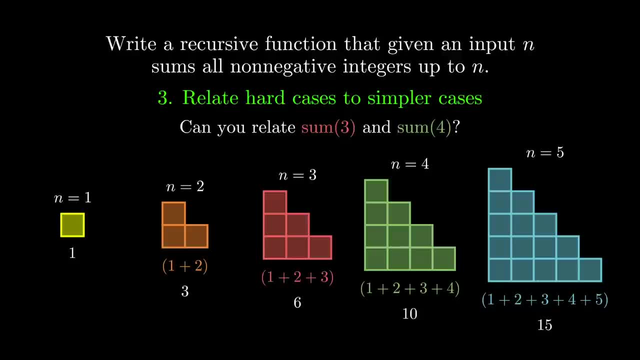 And similarly, if we know the answer to the n equals 3 case, we can get the answer to the n equals 4 case by adding 4.. And it's not too hard to convince yourself that this should be true in general, But, if necessary, feel free to try some larger cases to verify. 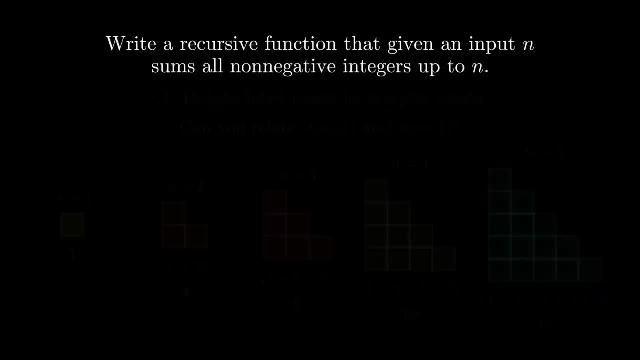 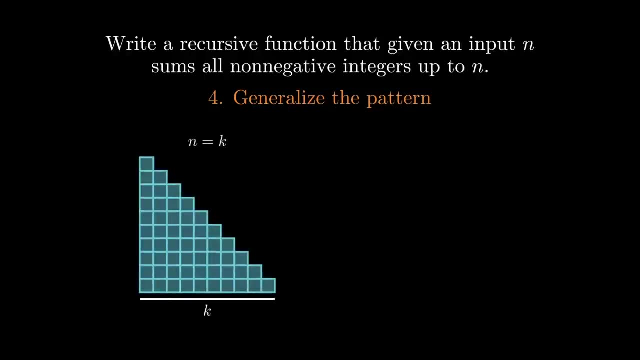 This now brings us to the fourth step, Key step, which is to generalize this pattern. Let's say we want to figure out the sum for the input: n equals k. We can find the sum by first taking the sum up to: n equals k minus 1.. 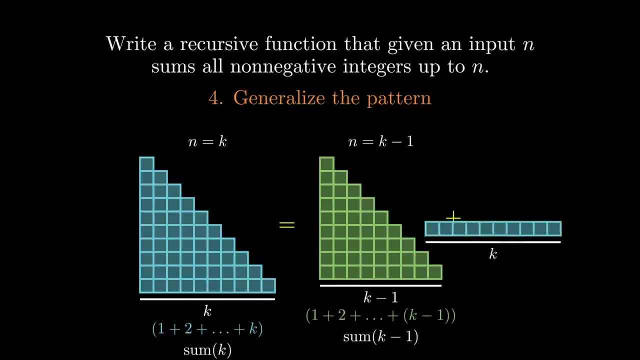 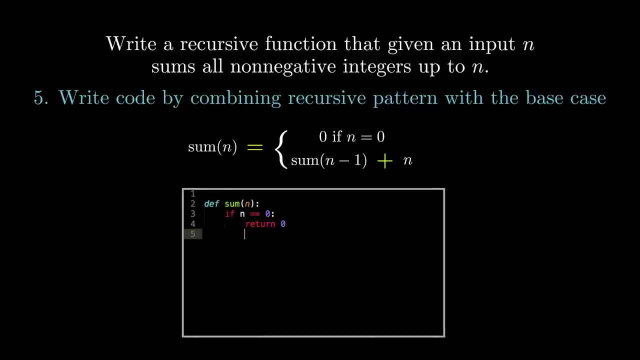 And then all we have to do is add k to this value, Once we've generalized the pattern. the last step now involves writing code by combining this recursive pattern with the base case. This actually turns out to be not too hard, Since the code almost writes itself from our base cases and recursive pattern. 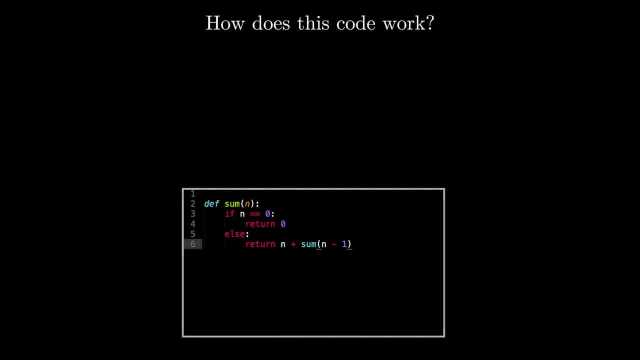 Let's dig a little bit deeper to see how this really works for a particular input. Let's say we run this function for input n equals 5.. What actually ends up happening? Well, we go through the initial function and then hit a recursive case. 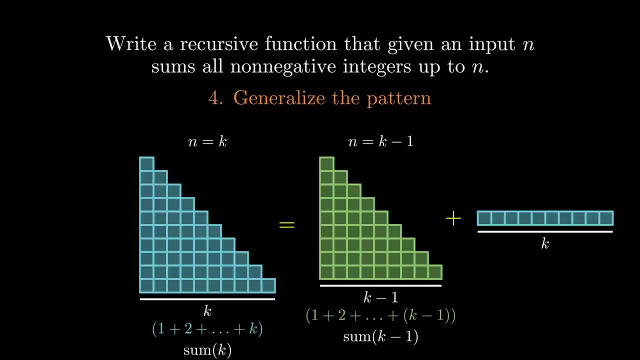 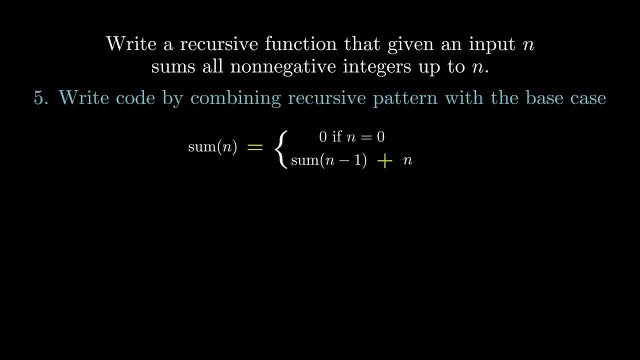 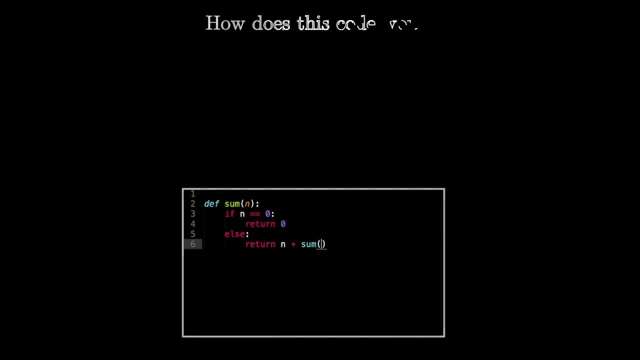 Once we've generalized the pattern, the last step now involves writing code by combining this recursive pattern with the base case. This actually turns out to be not too hard, Since the code almost writes itself from our base cases and recursive pattern. Let's dig a little bit deeper to see how this really works for a particular input. 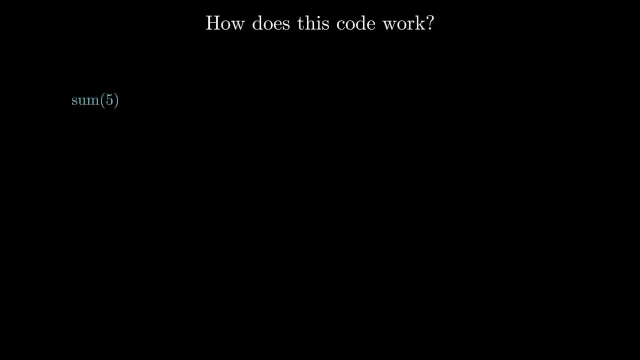 Let's say we run this function for input n equals 5.. What actually ends up happening? Well, we go through the initial function and then hit a recursive case which adds 5 to the result of calling our sum function on the input 4.. 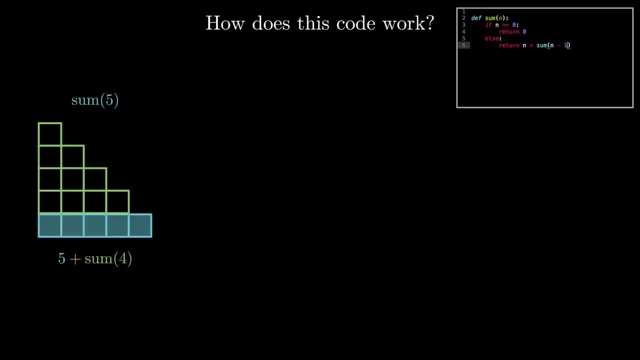 So we know that this should work. This should theoretically give us the value 10.. But technically this function hasn't been evaluated yet. What actually ends up happening is we have to go back into our function and repeat the process. We hit the recursive case again, which then causes us to now add 4 to the value of sum called on 3.. 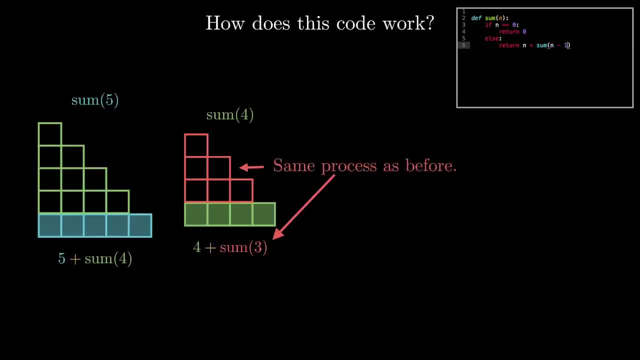 Which once again kicks off the same process as before. Let's take a moment to see how this unravels. This continues until we hit the base case, which then is used to solve the sum function called on n equals 1, which then solves the sum function called on n equals 2, and so on and so forth. 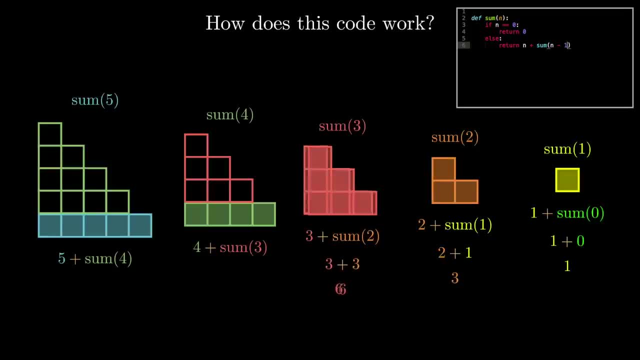 Until we eventually build up the solution for our original n equals 5 case. It's always okay to take some time To unravel the recursion to ensure that things work. But as you get more experience solving these type of problems, there's a concept called the recursive leap of faith that I would like you to think about. 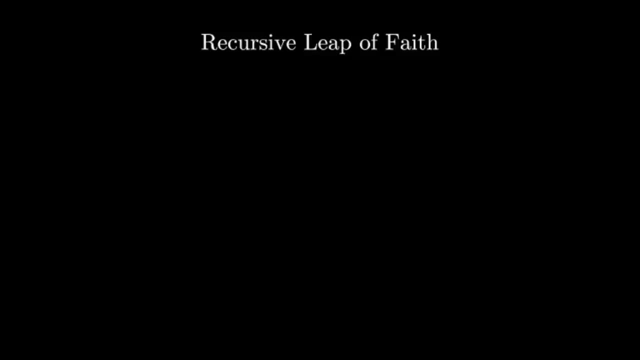 The recursive leap of faith makes solving recursive problems much faster. It's all about assuming that easier versions of the problem will be correct. In this particular problem, the recursive leap of faith would say that if I wanted to solve sum called on, n equals 5.. 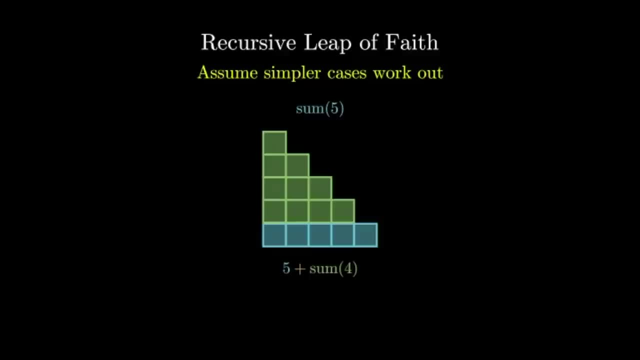 Let me just assume that sum on n equals 5 is going to solve the recursive leap of faith, And then if I add 5 to that sum called on, n equals 5 will also be correct. Don't worry if you're a little hesitant to believe in the recursive leap of faith. 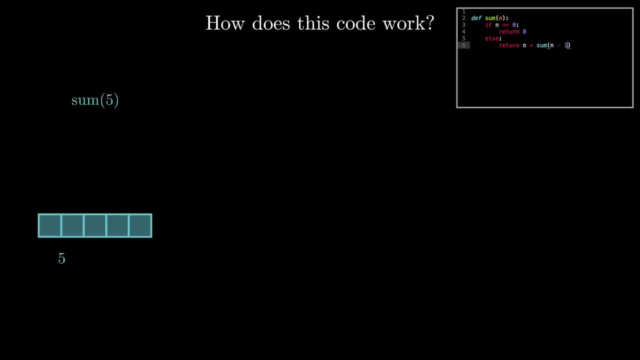 which adds 5 to the result of calling our sum function on the input 4.. So we know that this should work. This should theoretically give us the value 10.. But technically this function hasn't been evaluated yet. What actually ends up happening is we have to go back into our function and repeat the process. 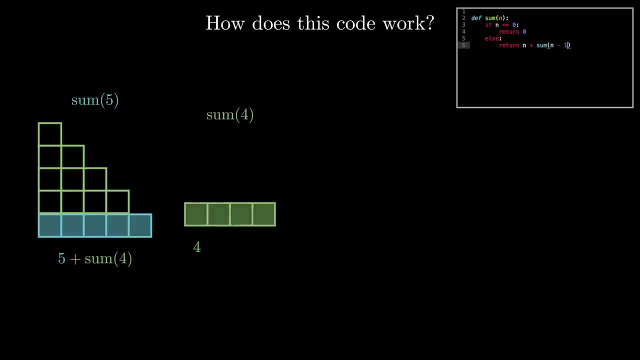 We hit the recursive case again, which then causes us to now add 4 to the value of sum, called on 3.. Which once again kicks off the same process as before. Let's take a moment to see how this unravels. This continues until we hit the base case, which then is used to solve the sum function called on. 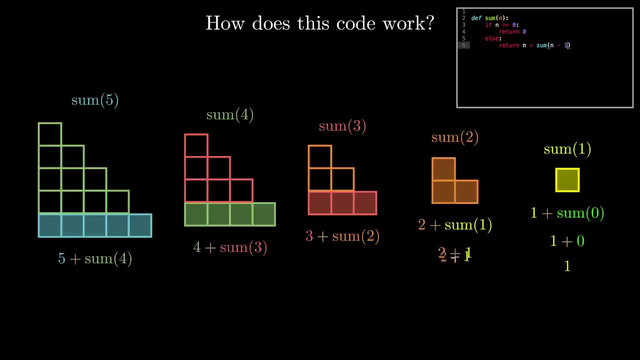 n equals 1, which then solves the sum function called on n equals 2, and so on and so forth, Until we eventually build up the solution for our original n equals 5 case. It's always okay to take some time To unravel the recursion to ensure that things work. 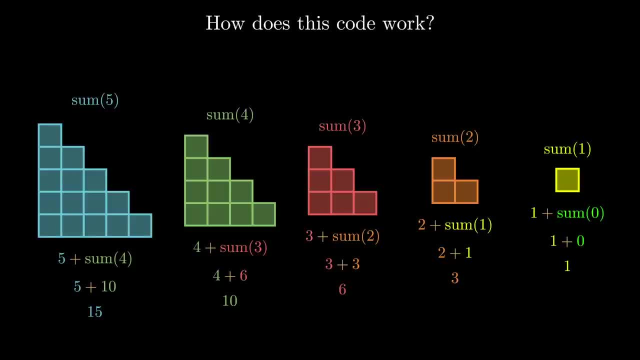 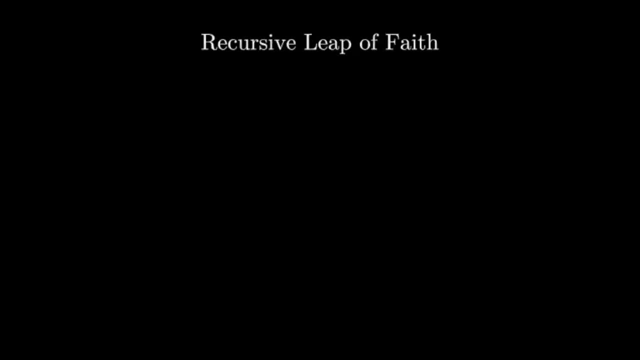 But as you get more experience solving these type of problems, there's a concept called the recursive leap of faith that I would like you to think about. The recursive leap of faith makes solving recursive problems much faster. It's all about assuming that easier versions of the problem will be correct. 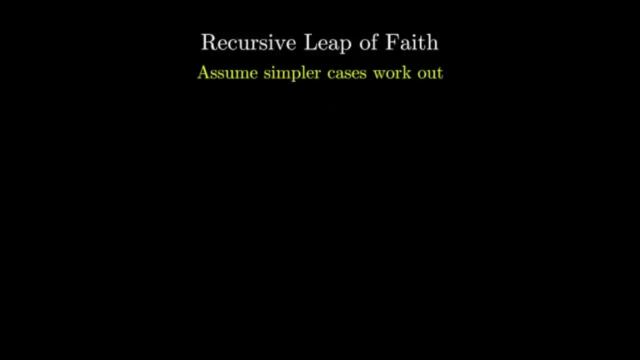 In this particular problem, the recursive leap of faith would say that if I wanted to solve sum called on n equals 5.. Let me just assume that sum on n equals 5 is going to solve the recursive leap of faith, And then if I add 5 to that sum called on, n equals 5 will also be correct. 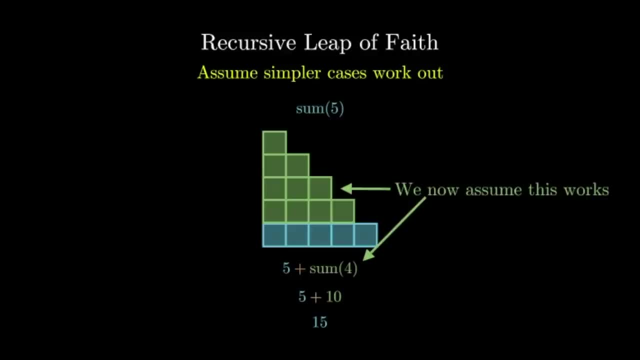 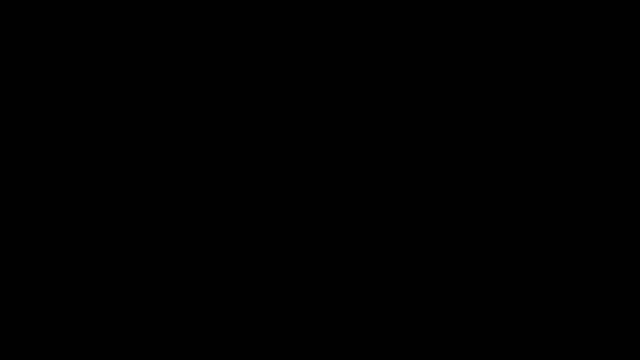 Don't worry if you're a little hesitant to believe in the recursive leap of faith, But it is a useful problem solving trick that helps in more complex recursive problems. Let's now explore a more involved recursive problem. Here's the problem: Write a function that takes two inputs, n and m- and outputs the number of unique paths from the top. 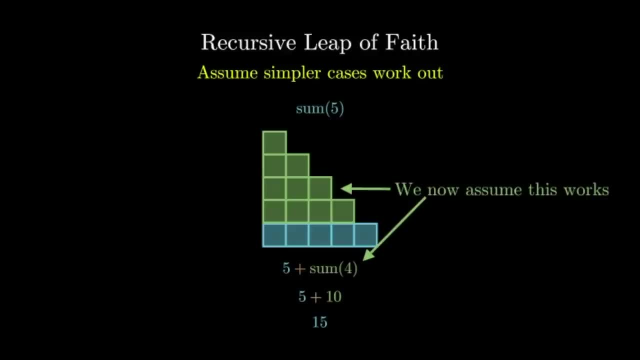 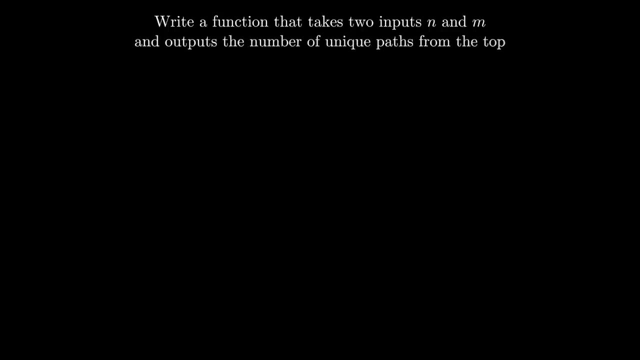 But it is a useful problem solving trick that helps in more complex recursive problems. Let's now explore a more involved recursive problem. Here's the problem: Write a function that takes two inputs, n and m, and outputs the number of unique paths from the top left corner to the bottom right corner of an n by m grid. 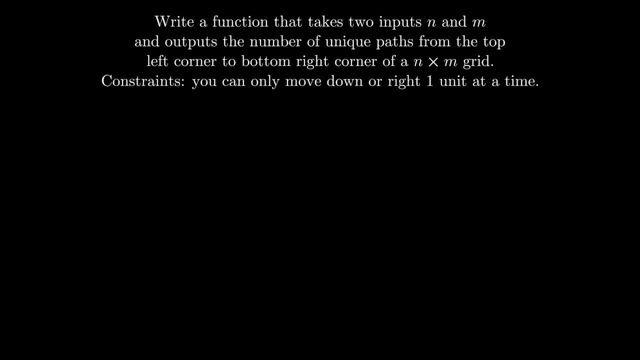 One key constraint is that you can only move down or right one unit at a time. Before we apply our five steps, let's first familiarize ourselves with a few inputs and outputs for this function. Here's what happens when n equals 2 and m is equal to 4.. 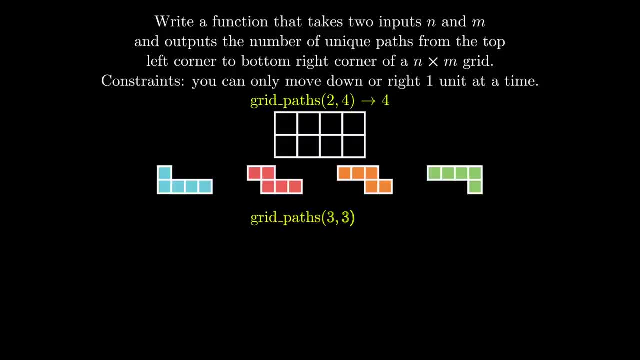 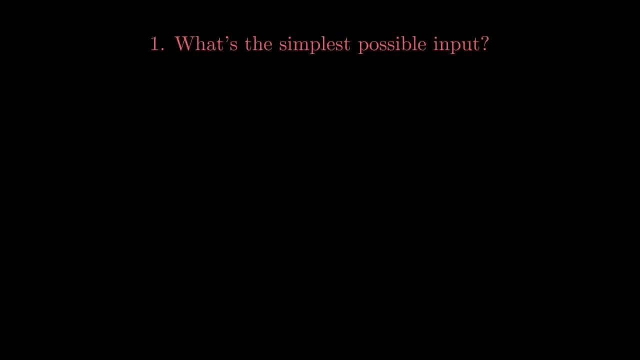 We end up with exactly four paths. And here's another example: with n equals 3 and m equals 3.. We end up with six unique paths. Alright, let's begin. Let's play around with some simple inputs and see what happens. The simplest possible reasonable input to this function is a one by one grid. 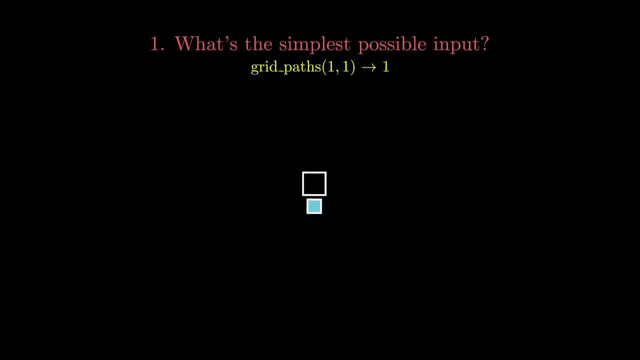 Where we end up with exactly one path. If we actually take a second to try some other simple inputs, you might notice something interesting. We can actually make a fairly comprehensive base case by noticing that if either one of these dimensions is going to be one, we have only one unique path. 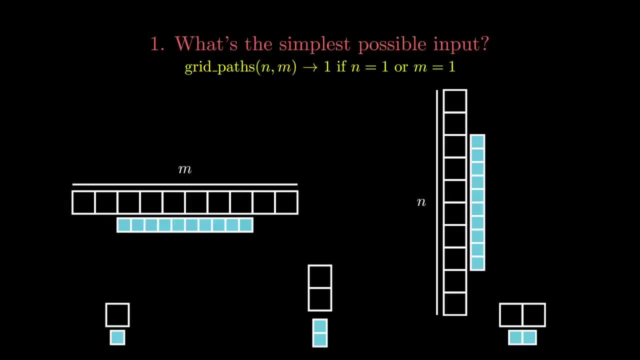 This can be written quite concisely as the following: base case. Often with base cases, you want to find a way to be as comprehensive as possible. Don't be afraid to adapt, though It's completely normal to come back later and modify the base case. 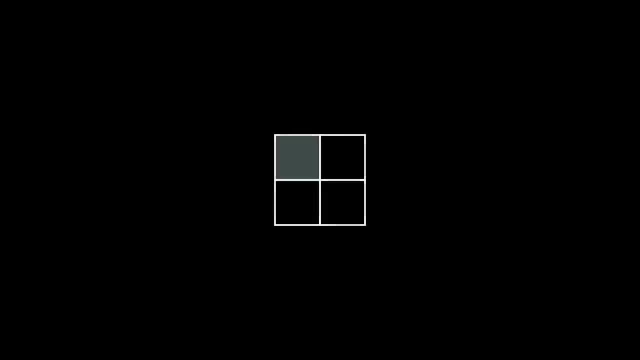 Let's now take a look at a decent sample size of examples to get a feel for the problem. When coming up with examples for recursive problems, it makes sense to do them in a sweeping manner where a lot of the examples are really close to each other. 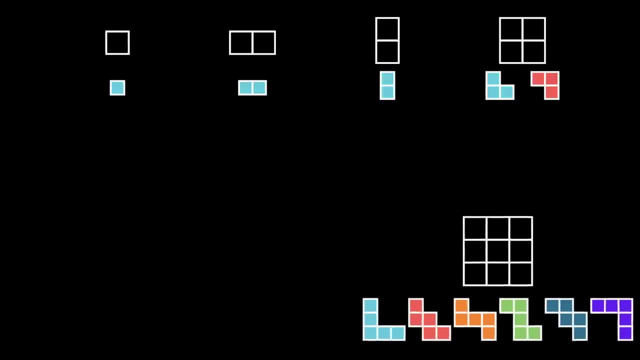 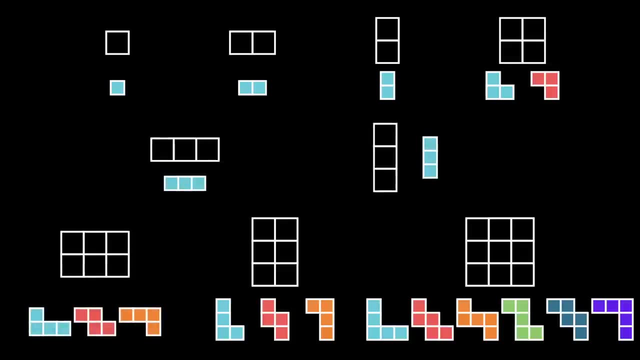 Remember, our ultimate goal is to find a way to solve any specific case using simpler versions of that case, so it makes sense to have examples that are close to each other. Alright, Now that we have a sizable set of examples, take a look at these and see if you notice any. 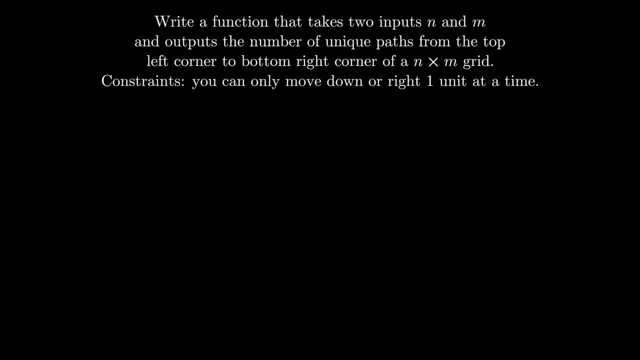 Left corner to the bottom right corner of an n by m grid. One key constraint is that you can only move down or right one unit at a time. Before we apply our five steps, let's first familiarize ourselves with a few inputs and outputs for this function. 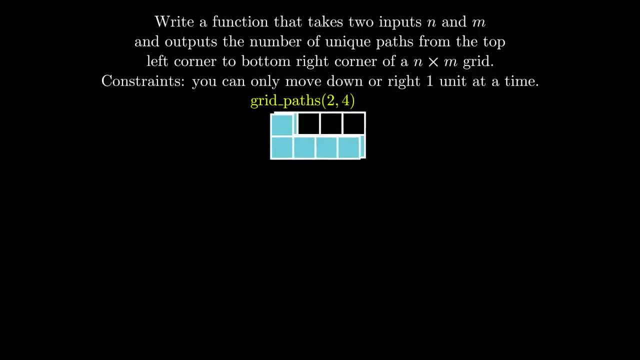 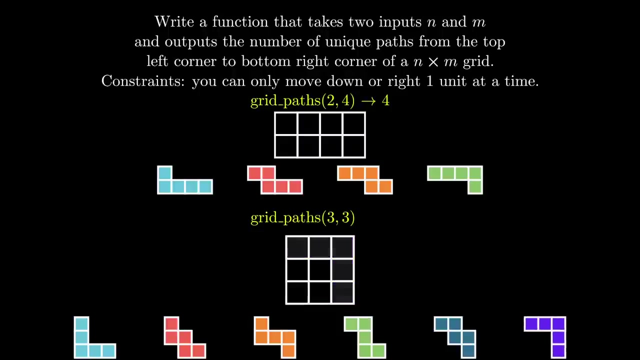 Here's what happens when n equals 2 and m is equal to 4. We end up with exactly four paths. Here's another example: with n equals 3 and m equals 3. We end up with six unique paths. Alright, let's begin. 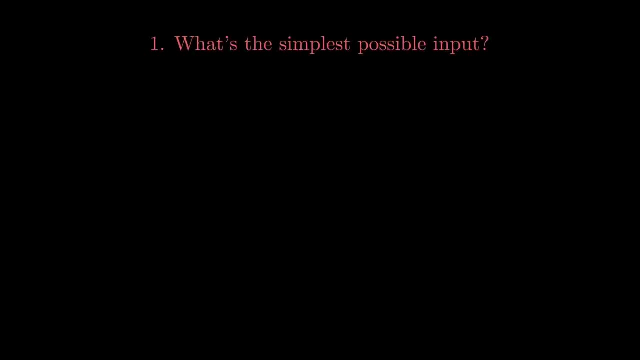 Let's play around with some simple inputs and see what happens. The simplest possible reasonable input to this function is a one by one grid, where we end up with exactly one path. If we actually take a second to try some other simple inputs, you might notice something interesting. 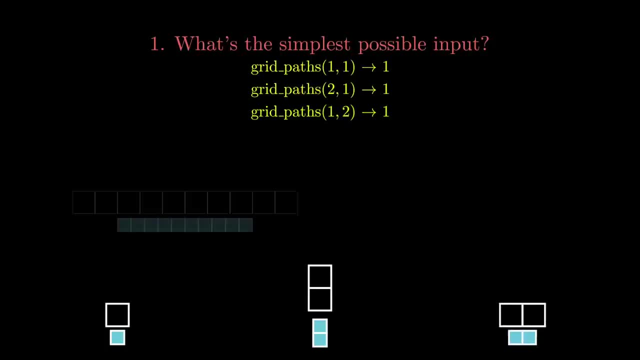 We can actually make a fairly comprehensive base case by noticing that if either one of these dimensions is going to be one, we have only one unique path. This can be written quite concisely as the following base case: Often with base cases, you want to find a way to be as comprehensive as possible. 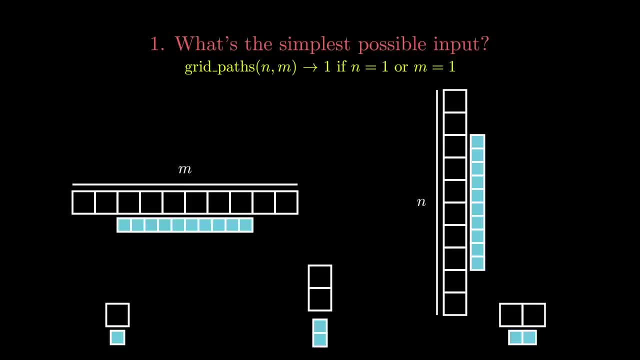 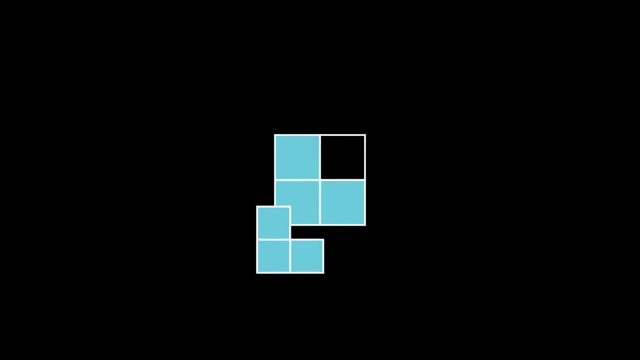 Don't be afraid to adapt, though It's completely normal to come back later and modify the base case. Let's now take a look at a decent sample size of examples to get a feel for the problem. When coming up with examples for recursive problems, it makes sense to do them in a sweeping 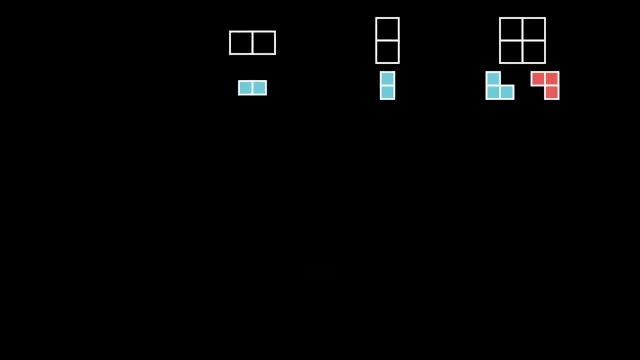 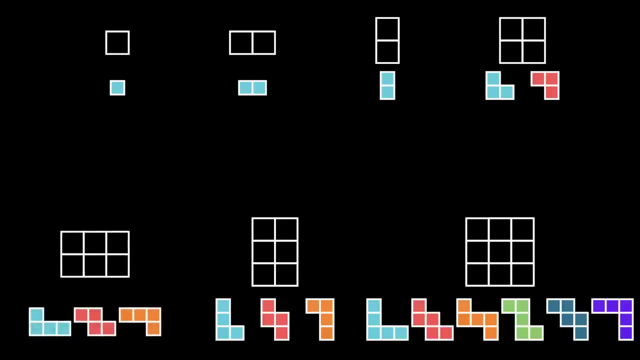 manner where a lot of the examples are really close to each other. Remember, our ultimate goal is to find a way to solve any specific case using simpler versions of that case, so it makes sense to have examples that are close to each other. Alright, Now that we have a sizable set of examples, take a look at these and see if you notice. 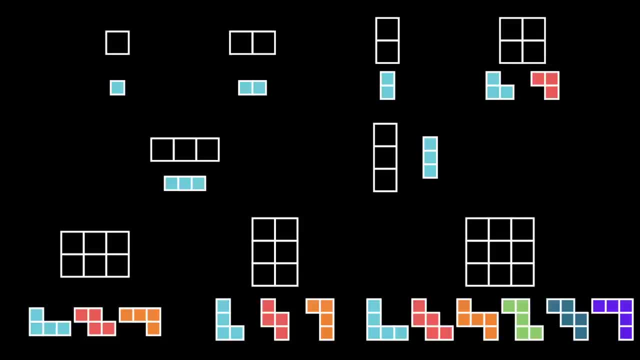 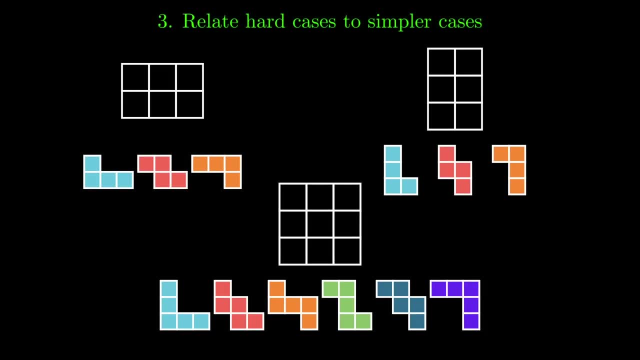 any interesting relationships between cases. I know that's a lot to look at, so as a hint, let's narrow down our focus to just these three examples. Do you notice anything? How about now? There's actually a really nice one-to-one correspondence between each path in the 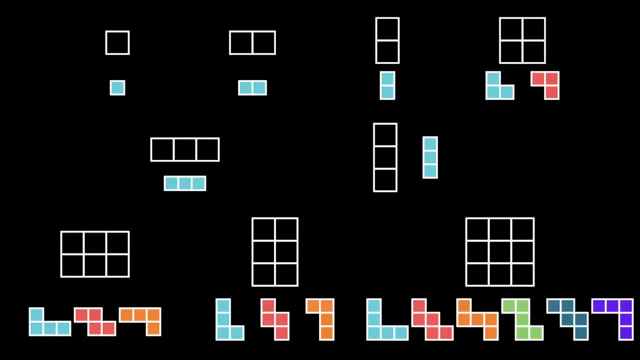 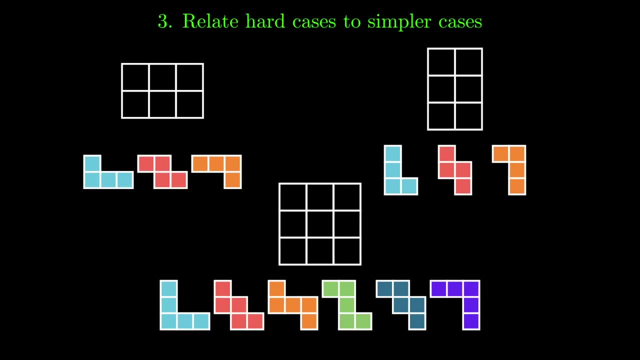 interesting relationships between cases. I know that's a lot to look at, so as a hint, let's narrow down our focus to just these three examples. Do you notice anything? How about now? There's actually a really nice one-to-one correspondence between each path in the. 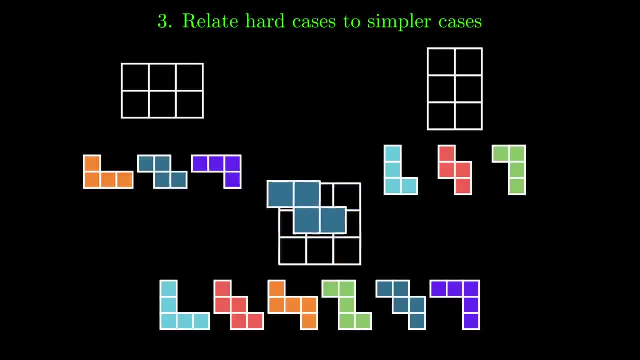 2x3 and 3x2 cases. to each path in the 3x3 case. For each path in the 2x3 case, we can take that path and go one unit down to create a path in the 3x3 case. 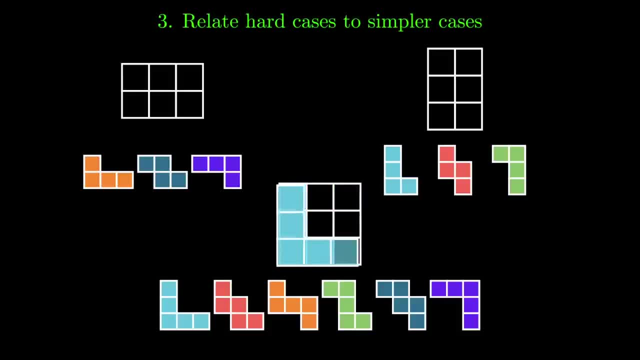 And for each path in the 3x2 case we can move one unit right to create a path in the 3x3 case. So at least in this example we can confidently say that the number of paths in the 3x3 example 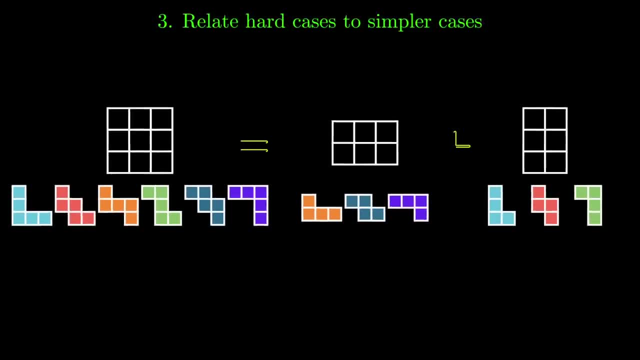 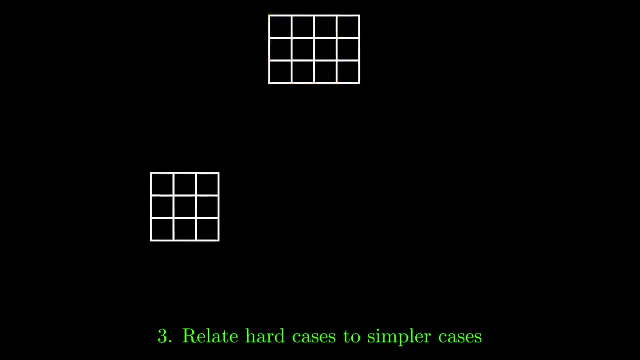 is the sum of the number of paths in the 2x3 example and the number of paths in the 3x2 example. But is that just a coincidence? Let's see if we can test this pattern by working backwards. Let's try to find the paths in the 3x4 case by analyzing a similar set of easier examples. 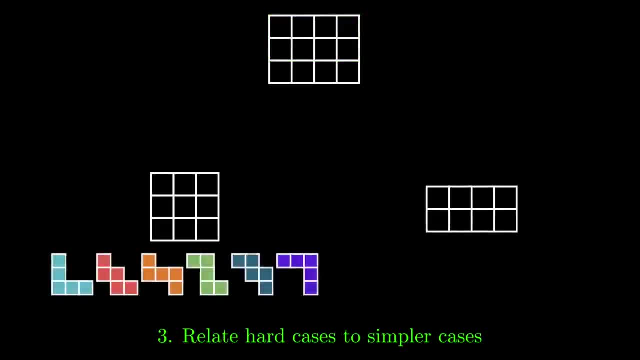 Following the earlier pattern, let's see if the number of paths in the 3x4 case is really the sum of the paths in the 3x3 case and 2x4 case. We'll take each path from the 3x3 case and move one to the right to make a corresponding path. 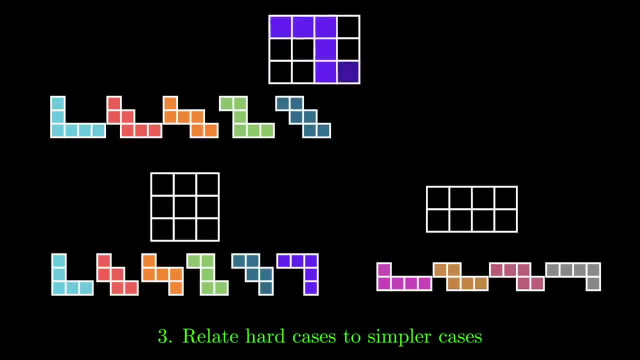 for the 3x4 case, And then we'll take each path in the 2x4 case and go one step down to make a path in the 3x4 case, And it turns out that the set of paths that are created from this construction. 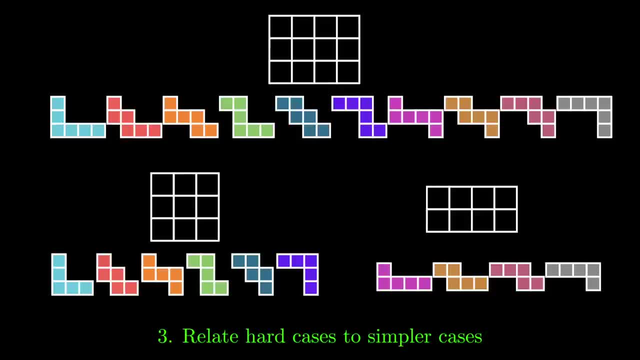 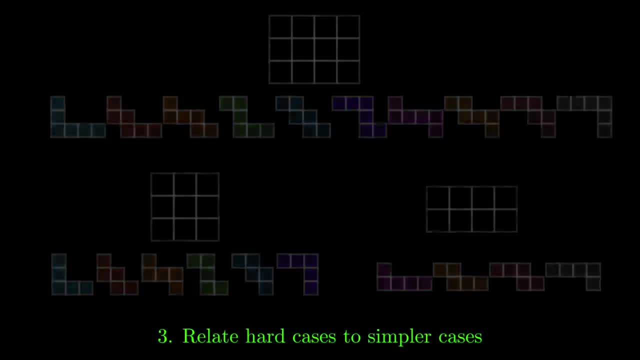 end up being all the unique paths through a 3x4 grid. Take a second to verify this for yourself if you're skeptical. So let's now generalize this pattern. We can find the total number of unique paths in an Nx4 case. 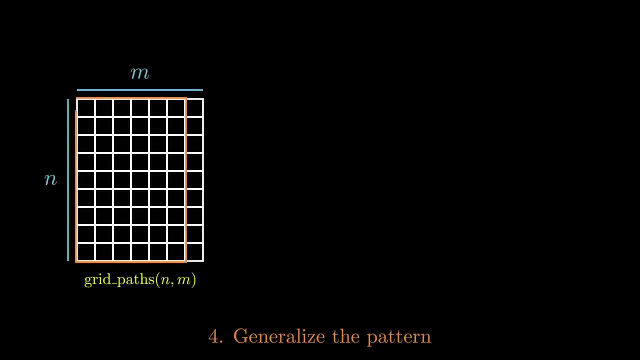 We can find the total number of unique paths in an NxM grid by first finding all the unique paths from the NxM-1 grid. Each of these paths correspond to a path in the NxM grid, since all we do is we move one unit to. 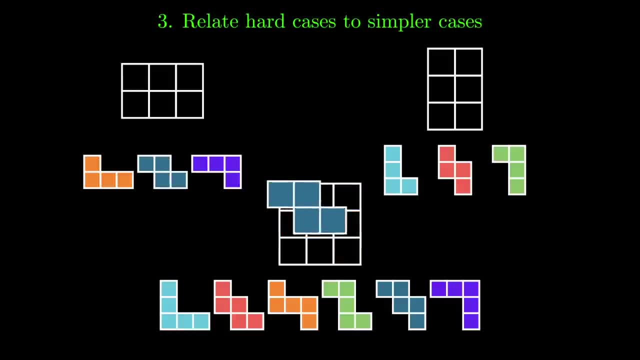 two-by-three and three-by-two cases to each path in the three-by-three case, For each path in the two-by-three case, we can take that path and go one unit down to create a path. in the three-by-three case, And for each path in the three-by-two case, we can move one unit right to create a path. 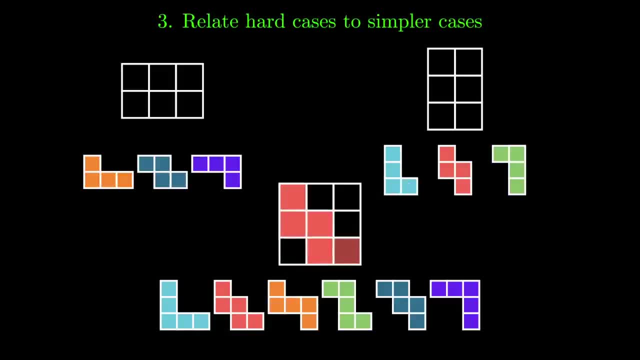 in the three-by-three case. So at least in this example we can confidently say that the number of paths in the three-by-three example is the sum of the number of paths in the two-by-three example and the number of paths in the three-by-two example. 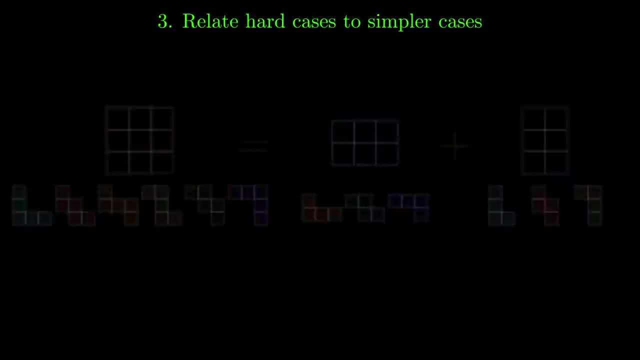 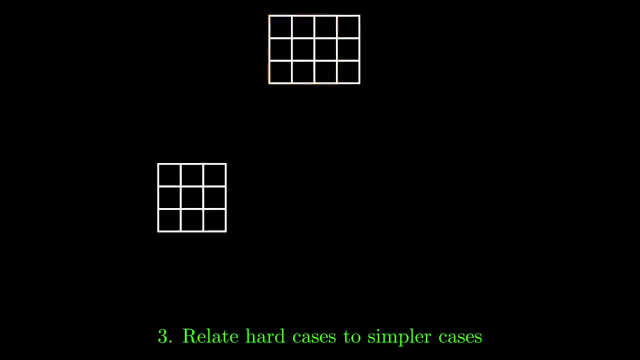 but is that just a coincidence? let's see if we can test this pattern by working backwards. let's try to find the paths in the 3x4 case by analyzing a similar set of easier examples following the earlier pattern. let's see if the number of paths in the 3x4 case is really the sum of the paths. 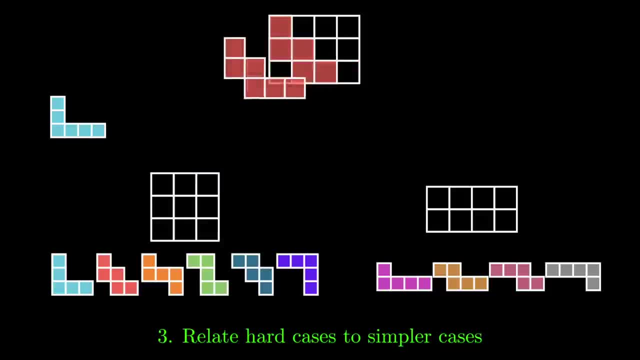 in the 3x3 case and 2x4 case. we'll take each path from the 3x3 case and move one to the right to make a corresponding path for the 3x4 case, and then we'll take each path in the 2x4 case and go. 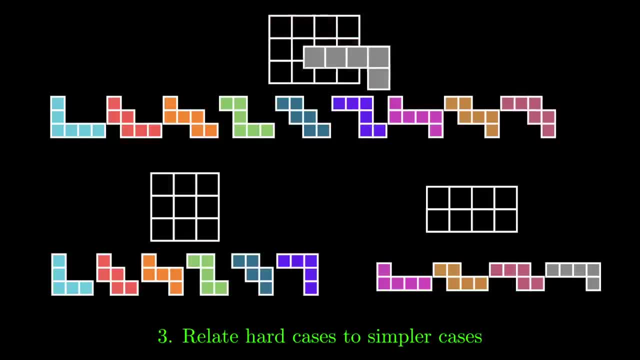 one step down to make a path in the 3x4 case, and it turns out that the set of paths that are created from this construction end up being all the unique paths through a 3x4 grid. take a second to verify this for yourself if you're skeptical. so let's now generalize this pattern. 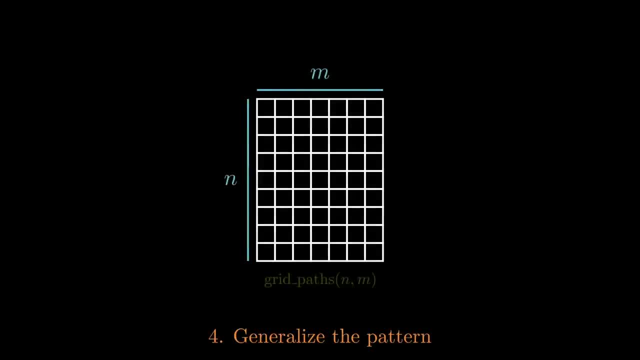 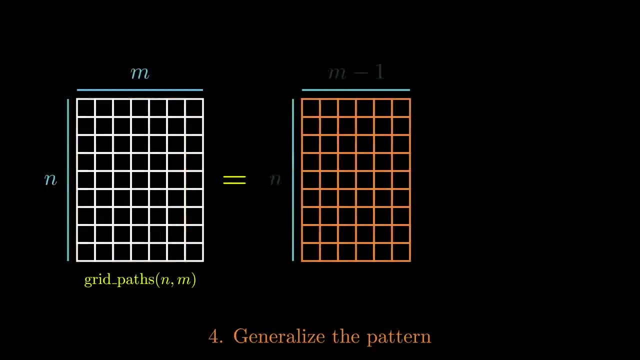 we can find the total number of unique paths in an n by m grid by first finding all the unique paths from the n by m, minus one grid. each of these paths correspond to a path in the n by m grid, since all we do is we move one unit to the right to create an associated path and the remaining 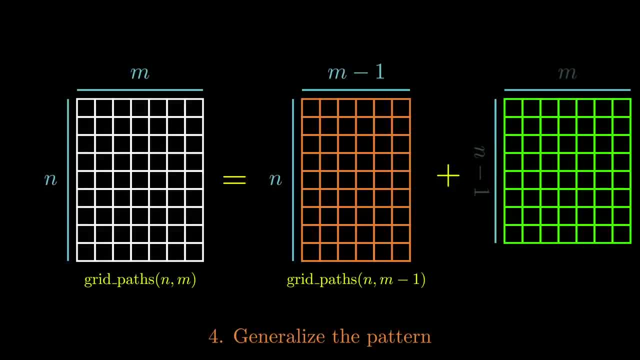 paths can be found by finding all the unique paths in an n minus one by m grid, where we now take each path, add one unit down and get the corresponding path in the n by m grid. we can then see that the path is now a 3x4 case. we can now take the path in the n by m grid and 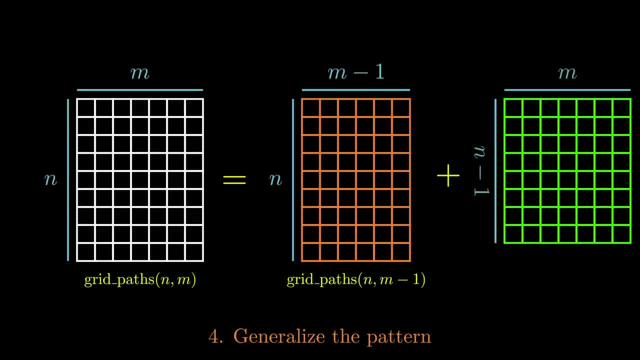 the right to create an associated path And the remaining paths can be found by finding all the unique paths in an N-1xM grid, where we now take each path, add one unit down and get the corresponding path in the NxM case. 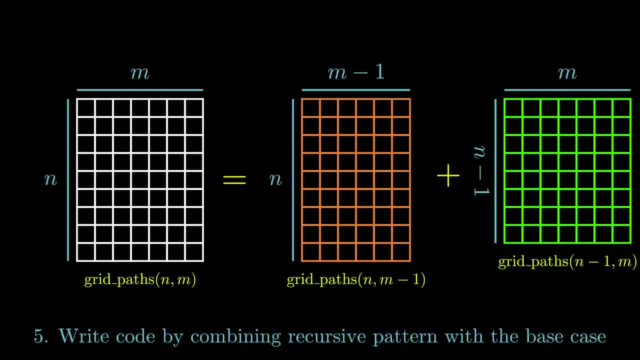 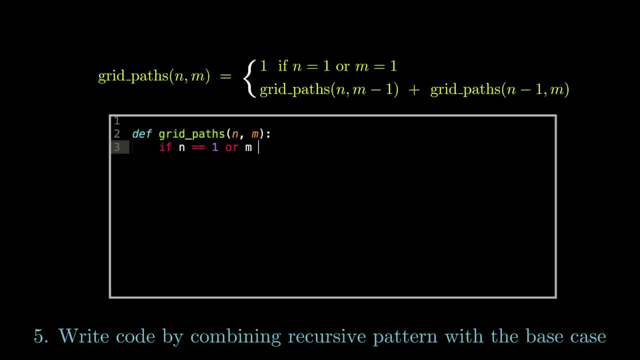 The last thing we do is take this general pattern, bring it together with the base case and now write code. The corresponding code for such a seemingly overwhelming problem ends up being remarkably simple and elegant, And you'll see this a lot in recursive problems. 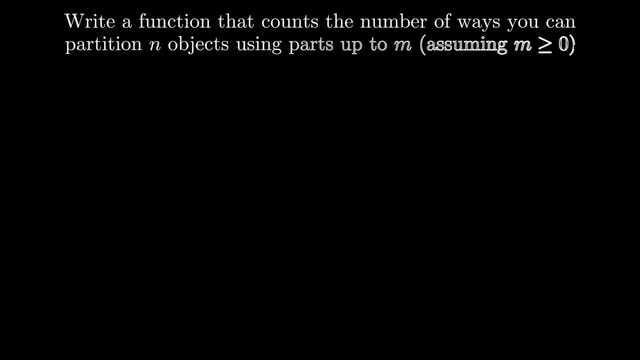 Speaking of hard problems, let's take a look at a really challenging problem. Here's the problem: Write a function that counts the number of ways you can partition N objects using parts up to M, As we've done so far. let's take a look at some examples to get a sense of what. 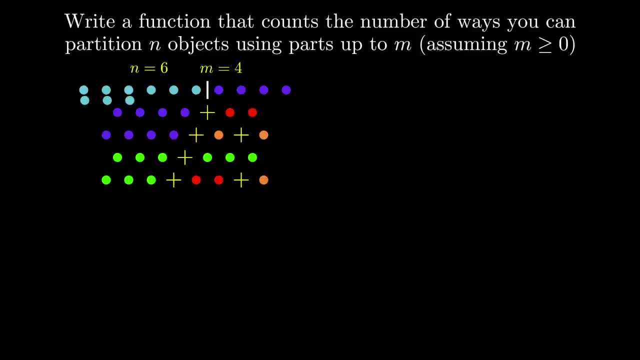 this problem is even asking For N equals 6 and M equals 4, here's how the partitions work out. We end up with a total of nine unique partitions. Let's take a look at one more example to make sure we really understand what's going on. 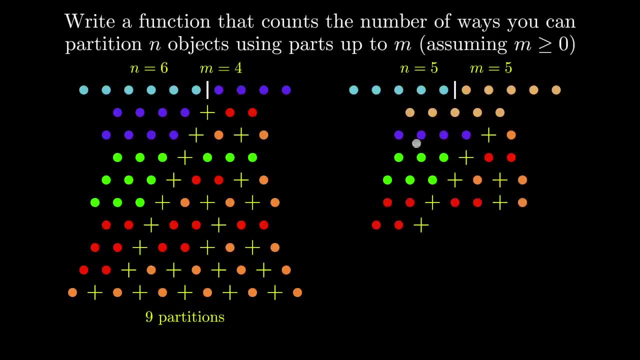 Here's what the partitions look like For inputs: N equals 5 and M equals 5.. Here we have seven unique partitions, And make sure you take a second to really understand why these are the only valid partitions. All right, so this problem definitely feels a little intimidating, since it's not really obvious. 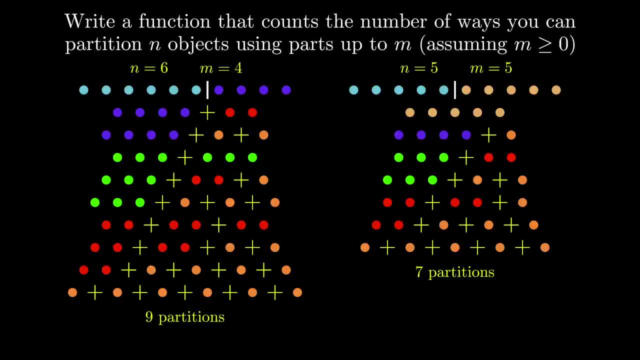 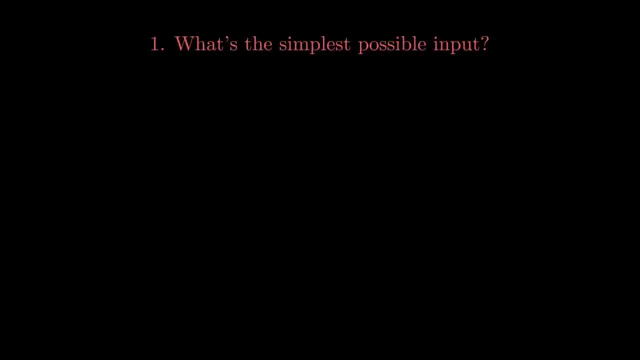 how we would even go about starting to solve it. But this is where we're going to have to fall back on our five steps. Let's start with step one. The first stop for what the simplest possible input should be, is when N is equal to zero. 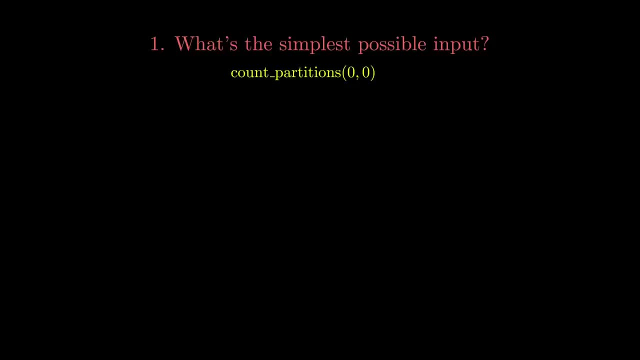 and M is equal to zero. What does this mean? It's asking you how many ways you can partition zero objects using parts up to zero. This may be a little bit mind blowing, but there's actually only one partition, and that partition is to include no parts and, in fact, trying inputs: N equals zero with M equals. 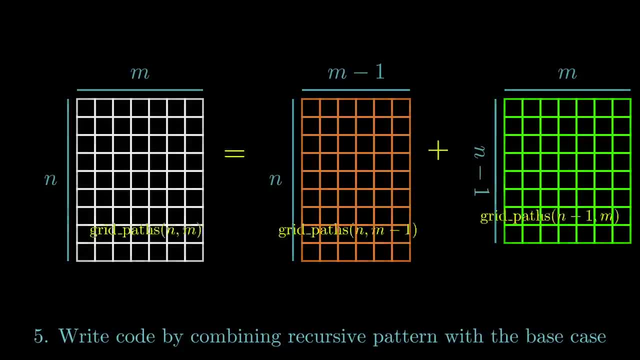 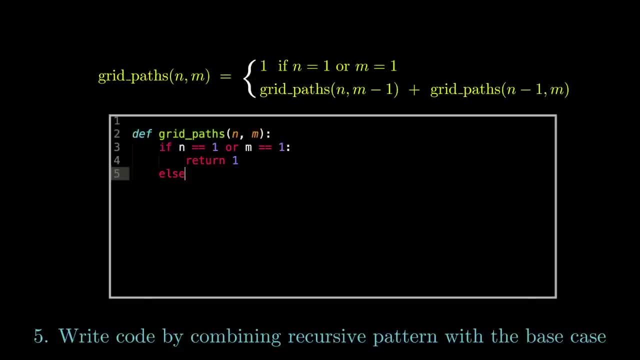 create a 3x4 case. once we've found this general relationship, the hard part is now over. the last thing we do is take this general pattern, bring it together with a base case and now write code. the corresponding code for such a seemingly overwhelming problem ends up being remarkably 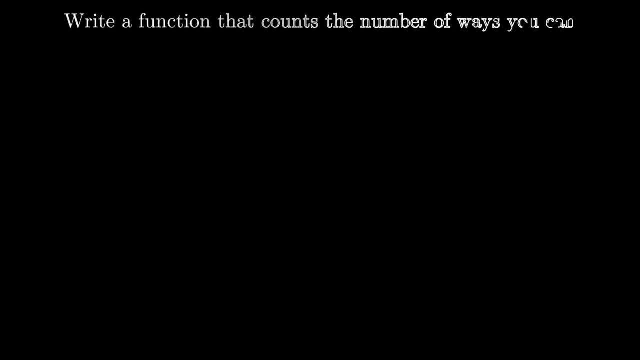 simple and elegant, and you'll see this a lot in recursive problems. speaking of hard problems, let's take a look at a really challenging problem: ways you can partition n objects using parts up to m, As we've done so far. let's take a look at 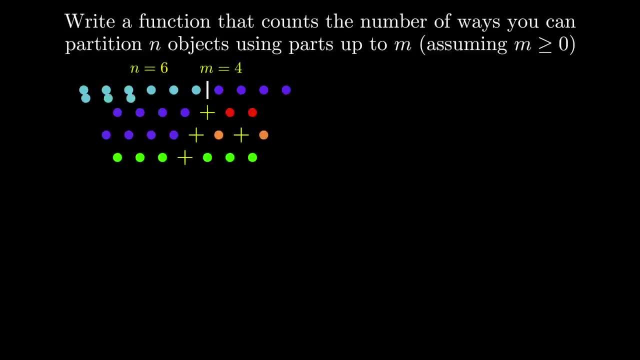 some examples to get a sense of what this problem is even asking For. n equals 6 and m equals 4, here's how the partitions work out. We end up with a total of 9 unique partitions. Let's take a look at one more example to make sure we really understand what's going on. Here's what the 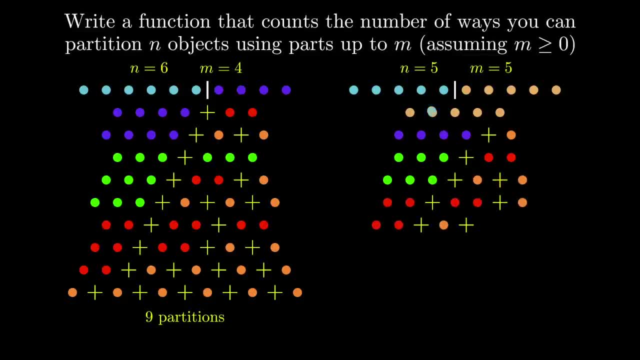 partitions look like for inputs: n equals 5 and m equals 5.. Here we have 7 unique partitions, and make sure you take a second to really understand why these are the only valid partitions. Alright, so this problem definitely feels a little intimidating, since it's not really obvious. 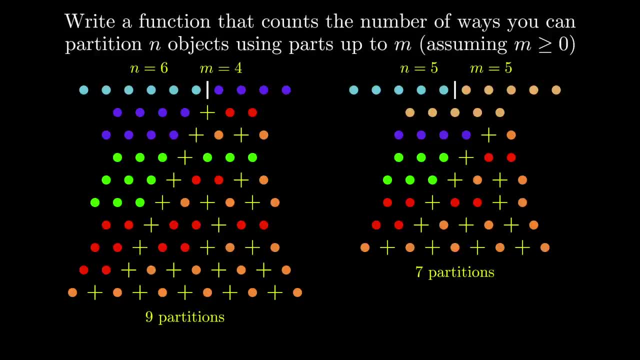 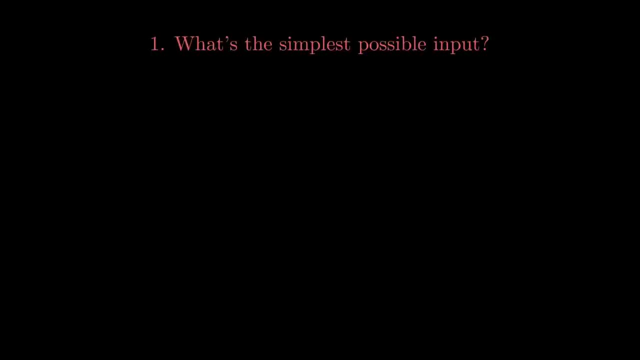 how we would even go about starting to solve it. But this is where we're going to have to fall back on our 5 steps. Let's start with step 1.. The first thought for what the simplest possible input should be is: when n is equal to 0 and m is: 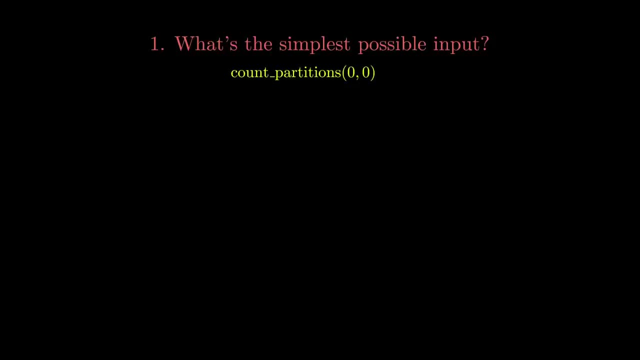 equal to 0.. But what does this mean? What it's asking is: how many ways can you partition 0 objects using parts up to 0.. This may be a little bit mind-blowing, but there's actually only one partition, and that partition is to include no parts. 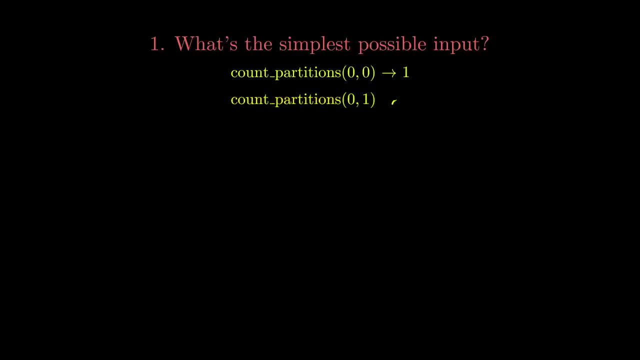 And in fact, trying inputs n equals 0 with m equals 1, and then n equals 0 with m equals 2, is really no different. This allows you to make another fairly comprehensive base case where the number of partitions is 1 if n is equal to 0. But there's some other simple. one, And then N equals zero. The simple way to do this is to give the same input a new partition, And that's how we solve the problem. Here's how you can do it. Number three: You can put the null components in the same order. 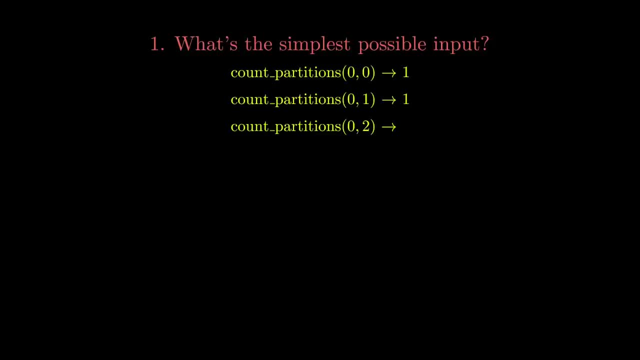 0 with m equals 2 is really no different. This allows you to make another fairly comprehensive base case where the number of partitions is 1 if n is equal to 0. But there's some other simple cases that we should also check out. 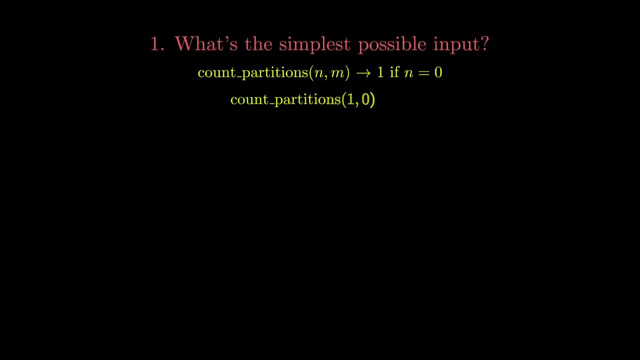 If n is equal to 1 and m is equal to 0, how many partitions do we have? How many ways can we partition one object if we are only allowed to use up to 0 parts? Well, this is actually impossible. We need at least one part. so there are 0 ways to partition these inputs. 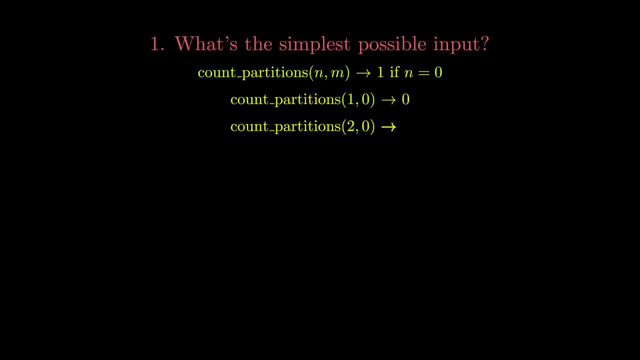 And the story stays the same, no matter what the n is. So this is the first example of a problem where we will need two separate base cases, the second one being that if m is equal to 0, we have 0 partitions. Alright, let's now visualize a sizable set of examples. 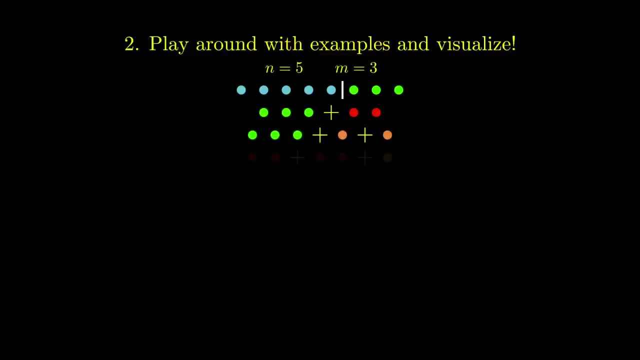 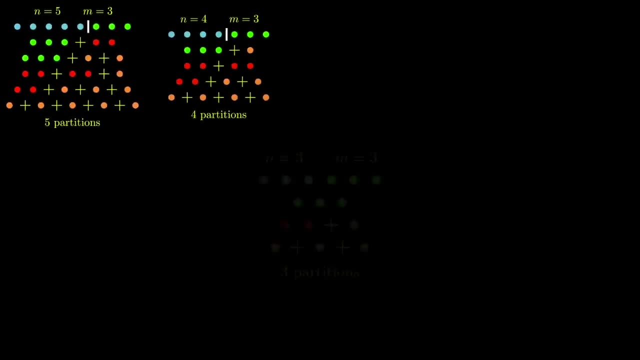 As before, let's look at examples that are relatively close to each other in numbers, so that it will make it easier for you. The problem is simple, but we can still solve it. Once again, if you're tasked to solving this problem, you don't want to be shy about. 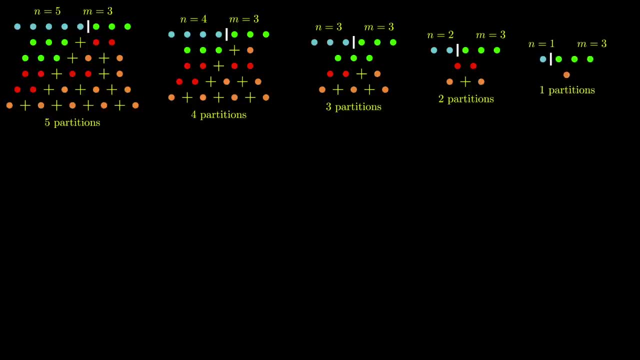 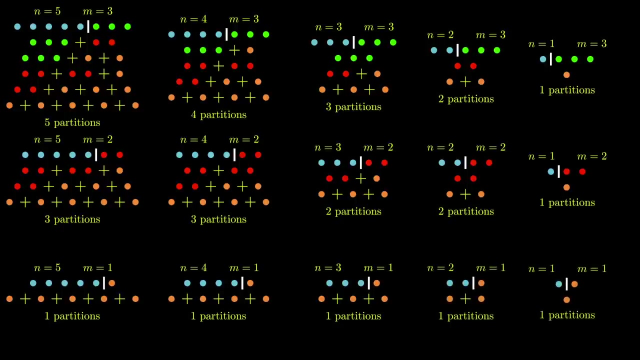 writing out a ton of examples. Not only will it make you more comfortable with the problem, but it also might help you find key insights to the solution. So, now that you have a good set of examples, take a moment to see if you notice any interesting. 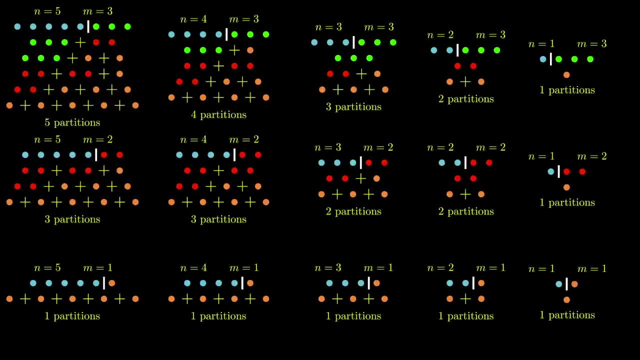 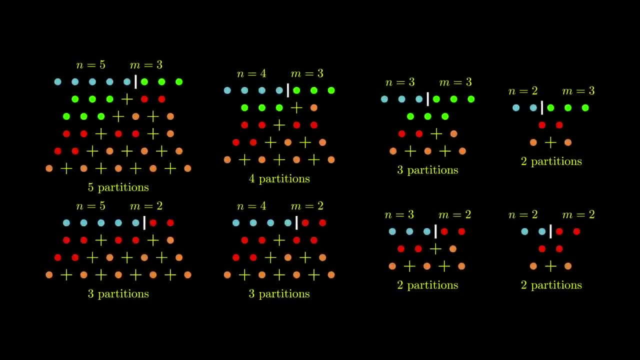 relationships among the partitions. Feel free to pause the video If you're struggling to find anything. let's narrow our focus to a subset of these examples. Alright, so the first interesting thing you might have noticed by looking at these examples is that a lot of the partitions on the larger problems are repeated in the easier version of the problem. 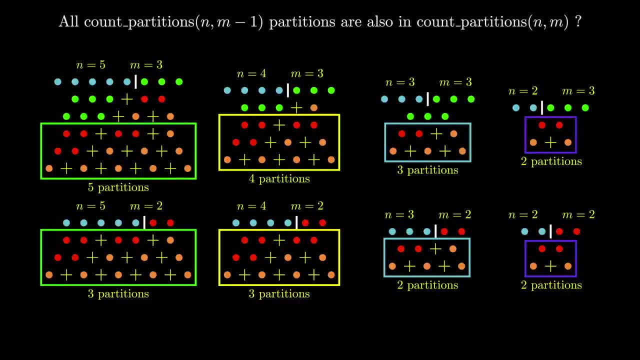 Isn't that a little bit wild? These are the types of patterns that show up a lot in these types of recursive problems and we definitely want to see if we can verify if this whole thing works. for larger examples, Let's take a look at the n equals 7, m equals 4 case. 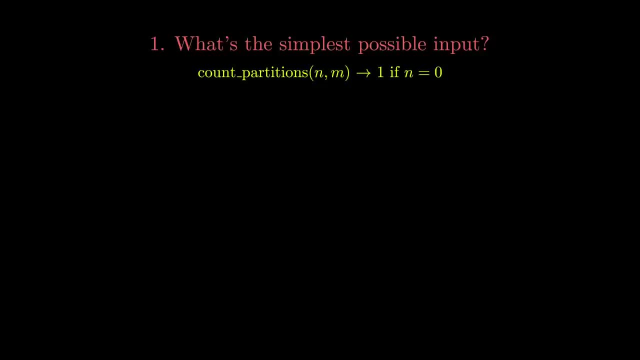 cases that we should also check out. If n is equal to 1 and m is equal to 0, how many partitions do we have? How many ways can we partition 1 object if we are only allowed to use up to 0 parts? Well, this is actually impossible. We need at least one part. 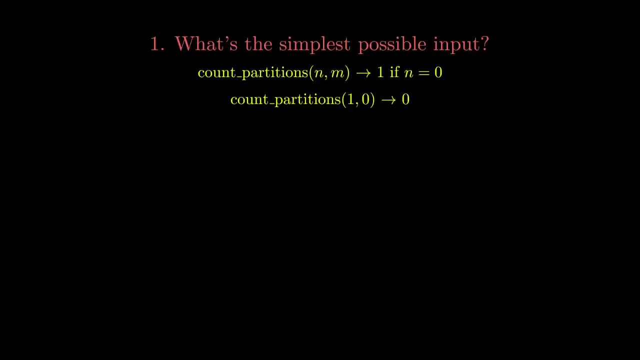 so there are zero ways to partition these inputs And the story stays the same, no matter what the n is. So this is the first example of a problem where we will need two separate base cases, the second one being that if m is equal to 0, we have zero partitions. 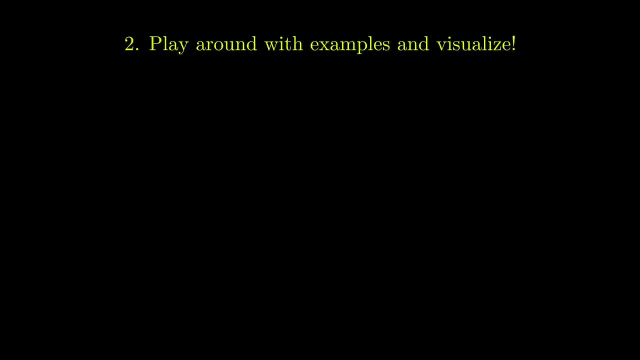 Alright, let's now visualize a sizable set of examples. As before, let's look at examples that are relatively close to each other in numbers, so that it will make it easier for us to find patterns in the following steps. Once again, if you're tasked to solving this problem, 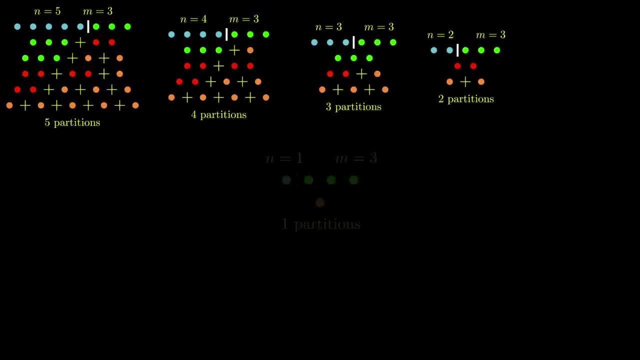 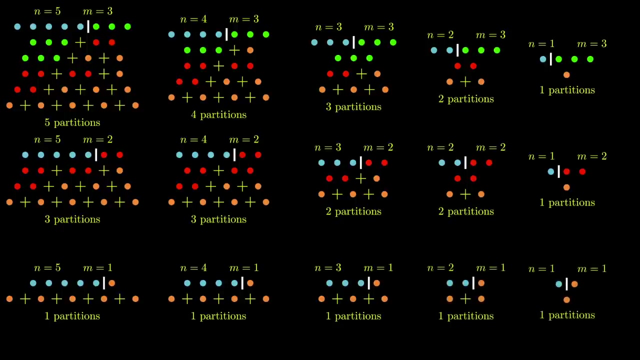 you don't want to be shy about writing out a ton of examples. Not only will it make you more comfortable with the problem, but it also might help you find key insights to the solution. So, now that you have a good set of examples, take a moment to see if you notice any. 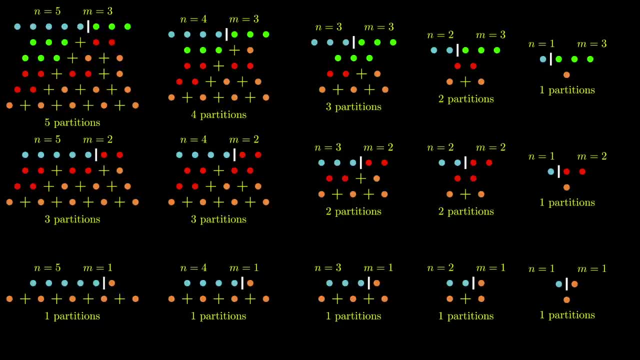 interest in finding patterns for the first set of examples. If it's a good set of examples, take a moment to see if you notice any interesting patterns in the following steps. relationships among the partitions. Feel free to pause the video If you're. 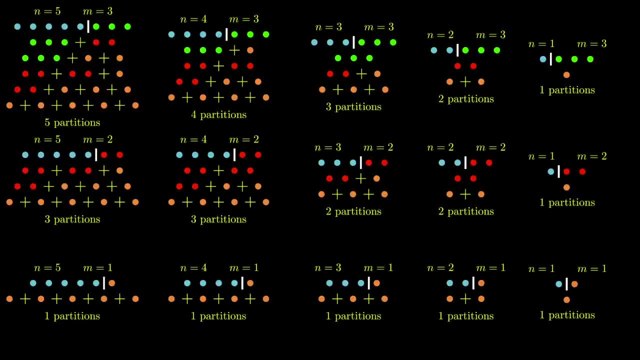 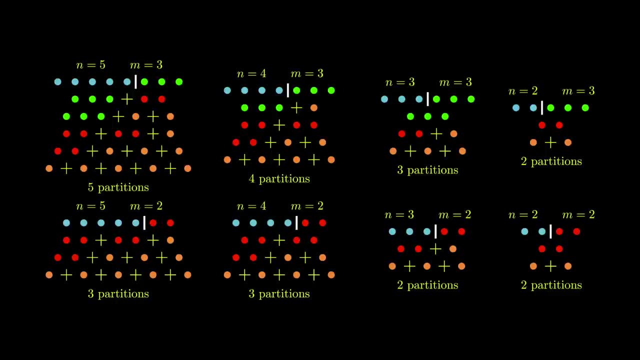 struggling to find anything. let's narrow our focus to a subset of these examples. Alright, so the first interesting thing you might have noticed by looking at these examples is that a lot of the partitions on the larger problems are repeated in the easier version of the problem. Isn't that a little bit wild? 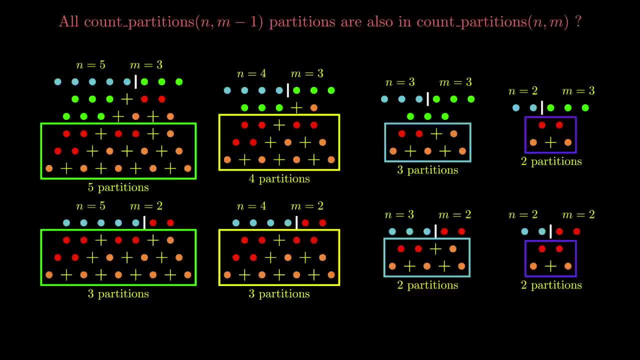 These are the types of patterns that show up a lot in these types of recursive problems and we definitely want to see if we can verify if this holds. for larger examples, Let's take a look at the n equals seven, m equals four case. We have a total of eleven partitions. So, going off our previous 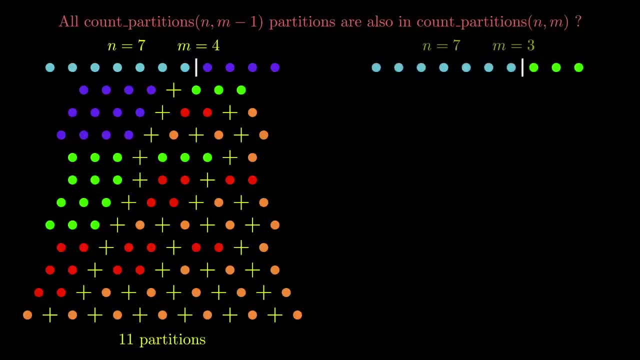 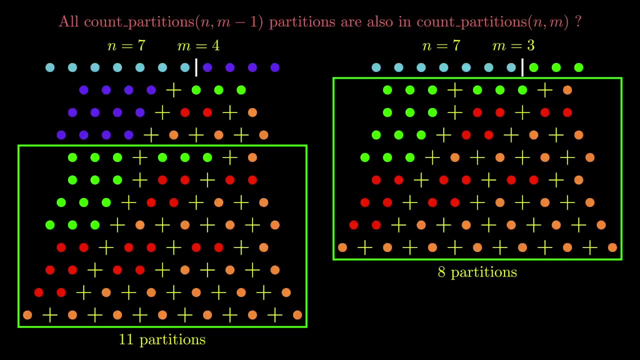 We have a total of 11 partitions. So, going off our previous example, we're expecting all the partitions of n equals 7, m equals 3 to show up in these partitions. And, in fact, when we go through the partitions, we indeed find that all eight partitions from the n. 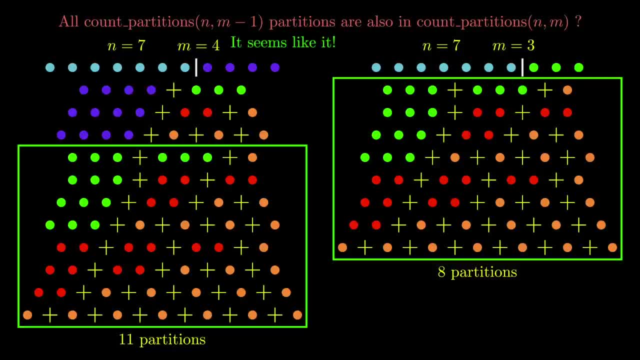 equals 7, m equals 3 case show up in the n equals 7, m equals 4 case. How in the world does that work? What crazy sorcery is going on here? The reason this happens is actually surprisingly simple If you take a moment to think about it from a perspective of how you are actually creating. 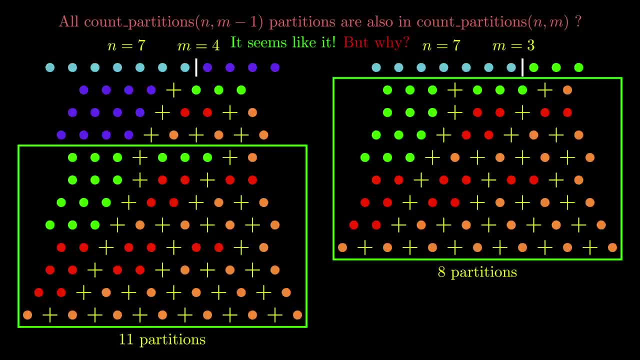 these partitions, you'll get an intuitive sense for why this is the case. When you're trying to partition 7 using parts up to 4, at some point this is going to include all the partitions of 7 using parts up to 3.. There's just no other way around it. More formally, we can assert that the partitions of n equals 7, m equals 3, m equals 4, m equals 3, m equals 3, m equals 4, m equals 4, m equals 5,, sum all sort of things. But this put an end to what we already were after class. 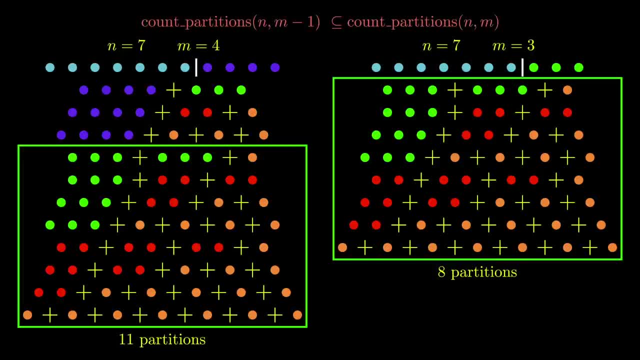 It seems that less substitutions of n operations bring greater McLangor hypothesis on what partitions of n can use parts up to m, less substitutions of n using parts up to l, and that all in line with the fact that these form rifles are essentially equal to the all. 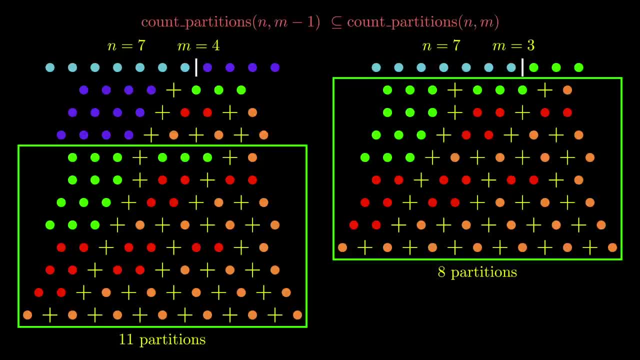 So at least twice as often as we usually assume if thisvadors enforce sometime same as the 25.. We'll get a future video on the miniburly partitions possibility too, but first let's head out of this ruler and move into a more cohesive fabric with some time to fold the. 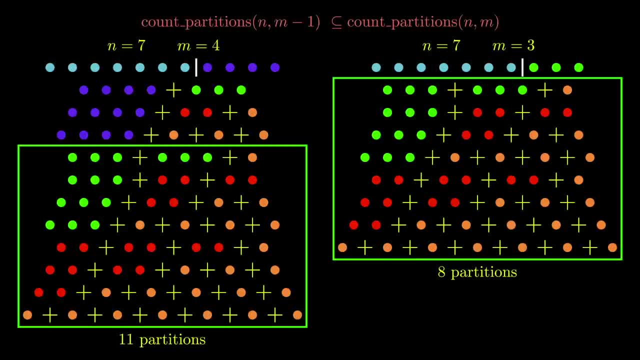 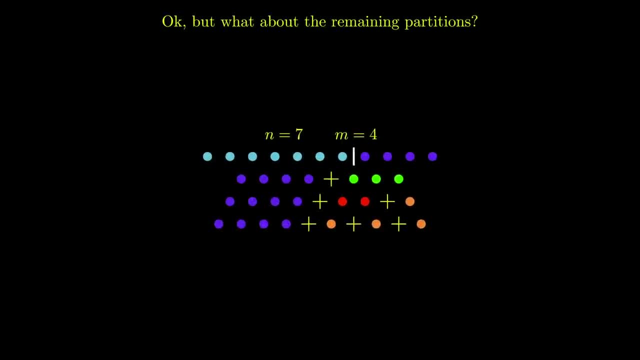 world. Now, before we dig into the history of the Artifacts, I think that being되는 less to which we are studying information could be really something we can have in some form of jargon-based journalism come from. Let's analyze these cases. What do they all have in common? Do you see it? 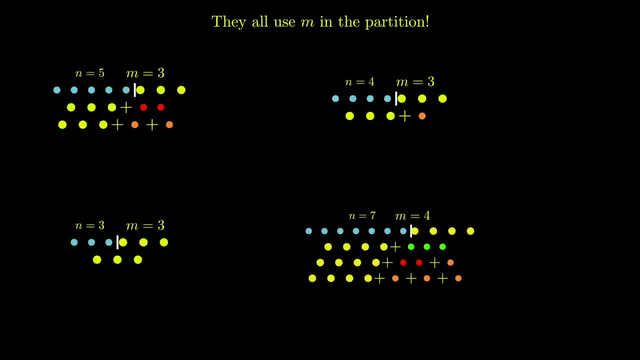 They all happen to use the actual m value as part of each partition, And this should make sense because the subsets that we removed were partitions of n using parts up to m minus 1.. So the partitions that are left here that use m represent the only other case. At this point, you might be thinking. 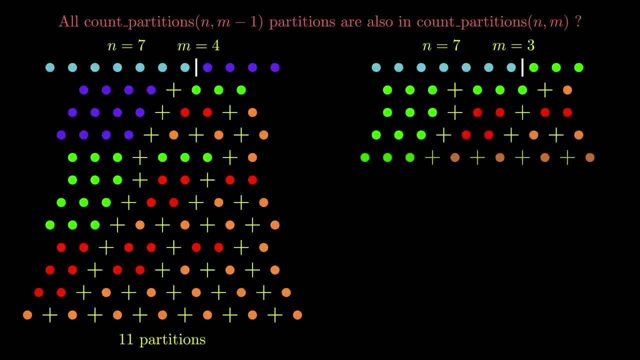 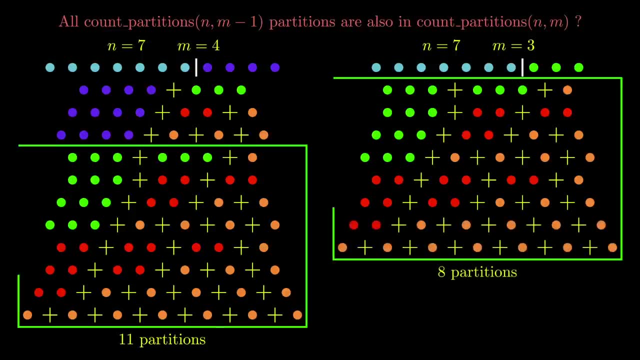 example, we're expecting all the partitions of n equals seven, m equals three to show up in these partitions. And in fact, when we go through the partitions, we indeed find that all eight partitions from the n equals seven, m equals three case show up in the larger example. 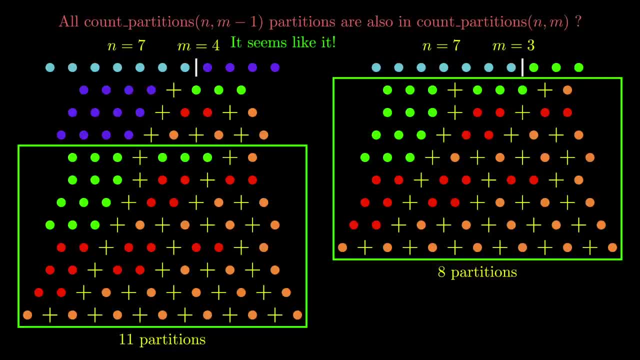 In the n equals seven, m equals four case. How in the world does that work? What crazy sorcery is going on here? The reason this happens is actually surprisingly simple. If you take a moment to think about it from a perspective of how you are actually creating these partitions, you'll get an intuitive sense. 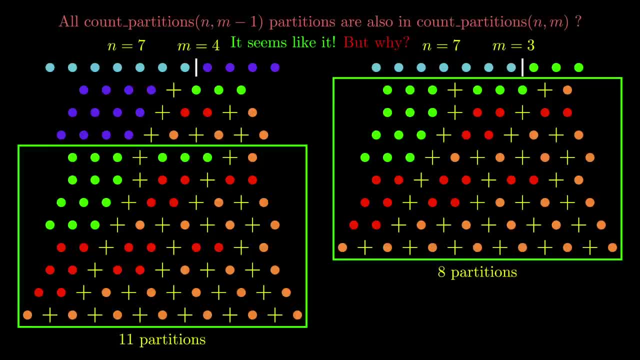 for why this is the case. When you're trying to partition seven using parts up to four at some point, this is going to include all the partitions of seven using parts up to three. There's just no other way around it. More formally, we can assert that the 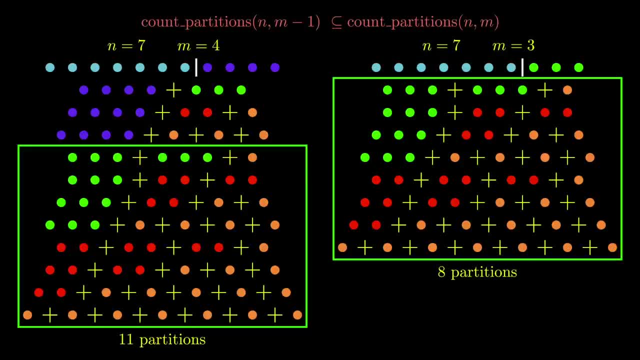 partitions of n using parts up to m minus one is a subset of the partitions of n using parts up to m. Okay, so this seems like a pretty good start. We now know that a subset of the partitions of n objects using parts up to m can be found from the simpler problem. 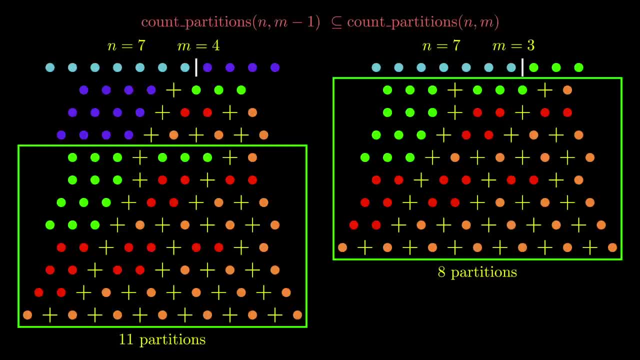 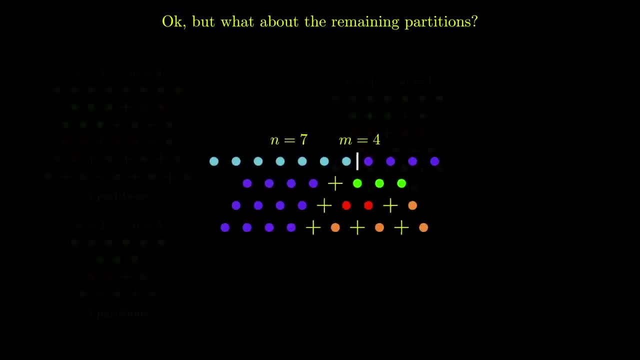 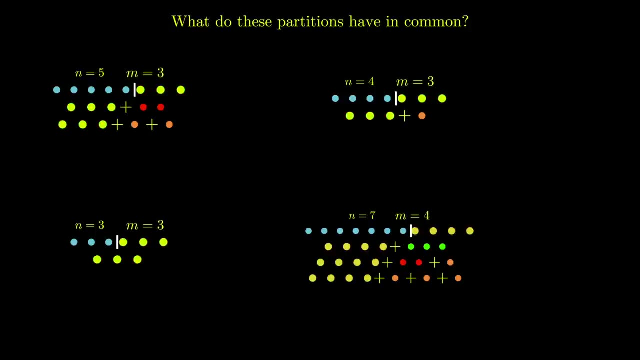 of partitioning n objects using parts up to m minus one. But what about the remaining partitions? Where do these partitions come from? Let's analyze these cases. What do they all have in common? Do you see it? They all happen to use the actual m value as part of each partition. 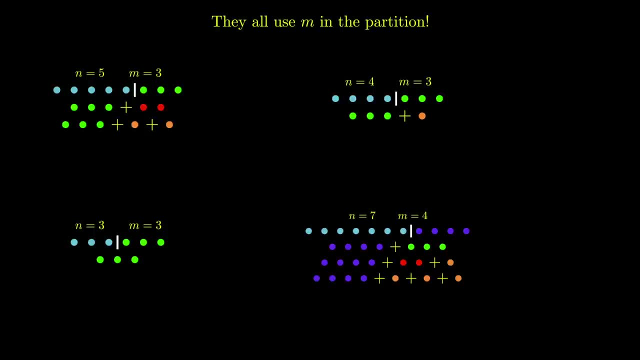 And this should make sense, because the subsets that we removed were partitions of n using parts up to m minus one. So the partitions that are left here that use m represent the only other case. At this point you might be thinking: okay, great, So the remaining? 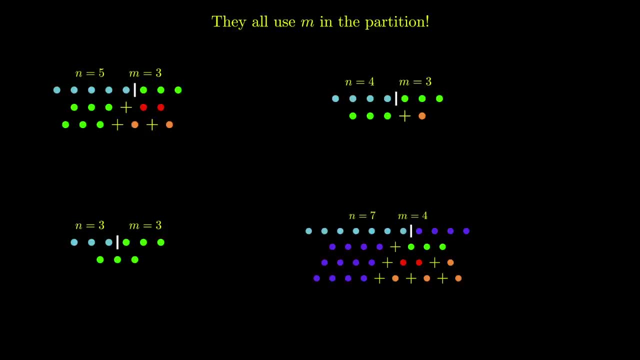 partitions all use m. How does this actually help us? Well, let's think about what it actually means to use m in a partition. Once we declare, hey, I'm going to go ahead and use m as a partition, this is what we end up having left in each of those cases. All that's going on here is we. 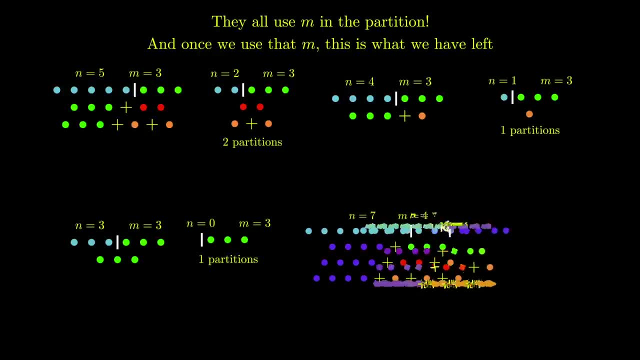 subtracted m from our original n objects. So we have a new n value with the same m value as before, And check this out. We have a new n value with the same m value as before, And check this out. We actually have another one to one correspondence If we add m to each. 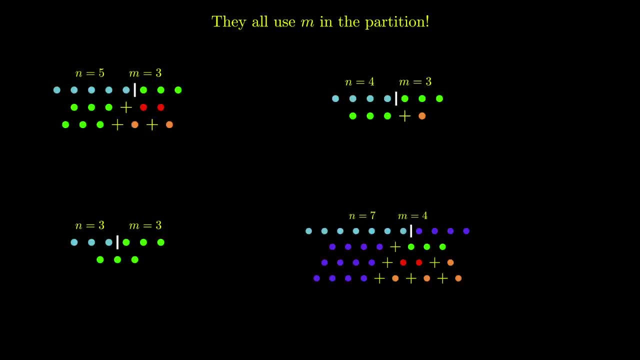 okay, great. So the remaining partitions all use m. How does this actually help us? Well, let's think about what it actually means to use m in a partition. Once we declare, hey, I'm going to go ahead and use m as a partition, this is what we end up having left in each of those cases All. 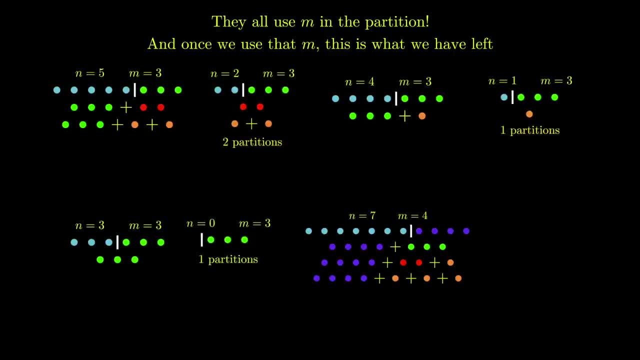 that's going on here is we subtracted m from our original n objects, So we have a new n value with the same m as a partition. So we have a new m as a partition. So we have a new m as a partition. 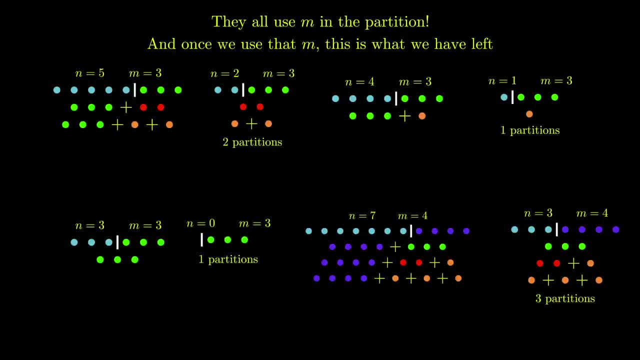 And check this out. We actually have another one-to-one correspondence. If we add m to each partition in the smaller problem, we end up with the same partition in our original problem. At this point you might still be a little skeptical, because we tried this only on relatively small. 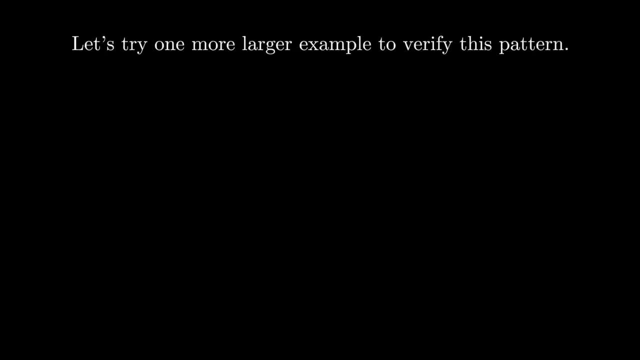 examples. So to really verify this, let's try one more large example, And this time we're going to try work backwards like we did in the grid problem. Let's look at the case where n is equal to 9 and m is equal to 5.. Let's try work backwards like we did in the grid problem. Let's look at the case. 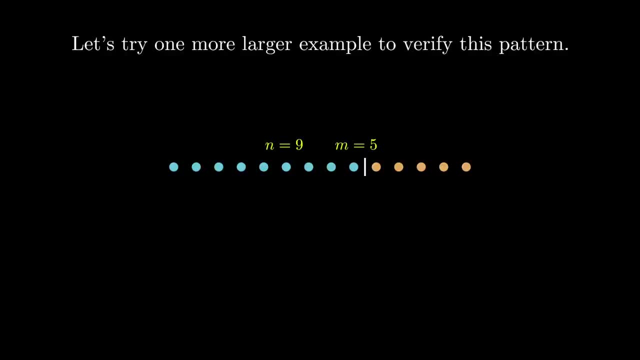 where n is equal to 9 and m is equal to 5.. Based on our current observations, we expect all the partitions in this case to correspond to the partitions in the n is equal to 4 and m is equal to 5 case. And then the n is equal to 9 and m is equal to 4 case. Remember the first subproblem? 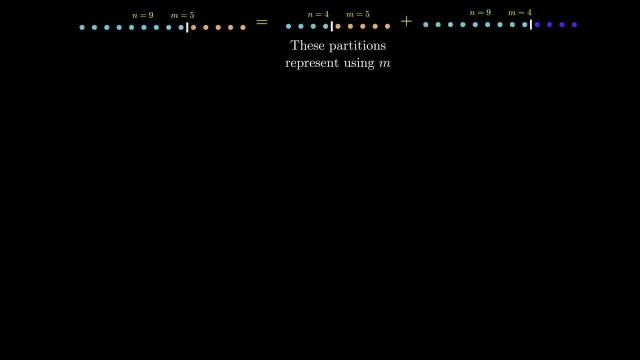 represents all the partitions that use our original m as part of the partition, And the second subproblem represents partitions that use parts up to m minus 1.. Here are the partitions, for m is equal to 4 and m is equal to 5 case. By adding m to each of these partitions, we generate the 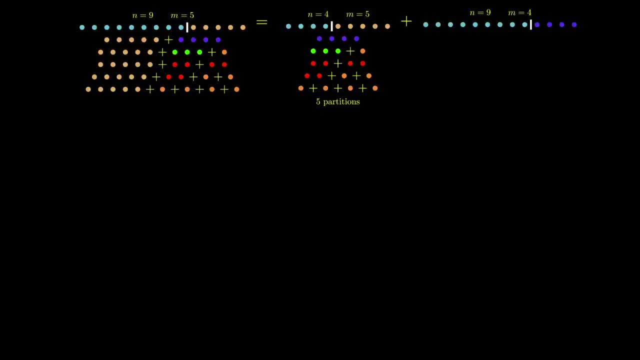 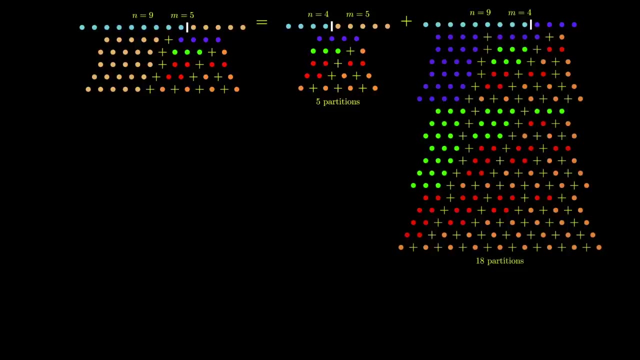 corresponding subset of partitions for the n is equal to 9 and m is equal to 5 case, And combining this with the 18 partitions from the n is equal to 9 and m is equal to 4 case. we end up with 23. 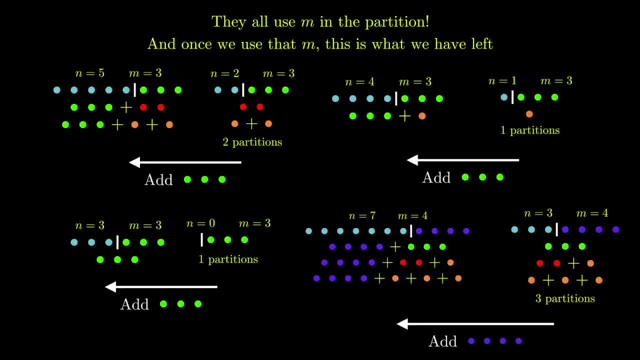 partition in the smaller problem, we end up with the same partition in our original problem. At this point you might still be a little skeptical, because we tried this only on relatively small examples. So to really verify this, let's try one more large example And this: 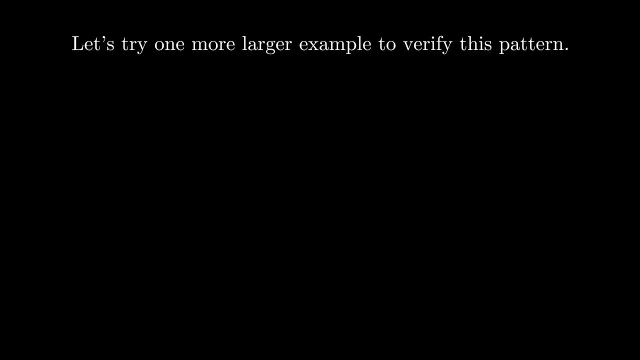 time we're going to try work backwards like we did in the grid problem. Let's look at the case where n is equal to nine and m is equal to five. Based on our current observations, we expect all the partitions in this case to correspond to the partitions in the n is equal. 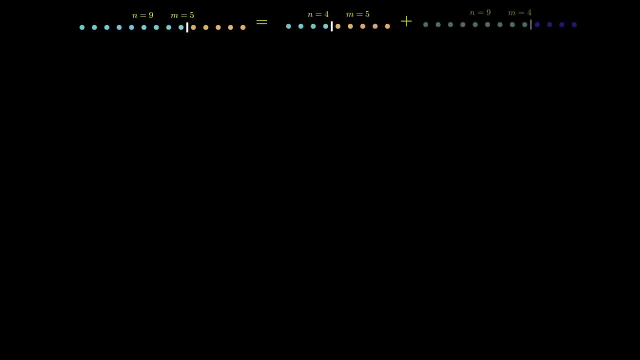 to four and m is equal to five case. And then the n is equal to nine and m is equal to four case. Remember, the first subproblem represents all the partitions that use our original m as part of the partition, And the second subproblem represents partitions that use: 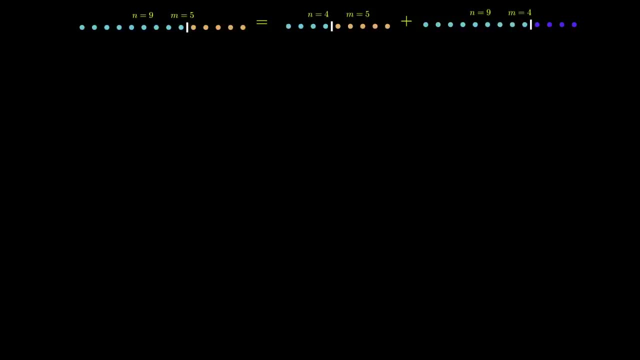 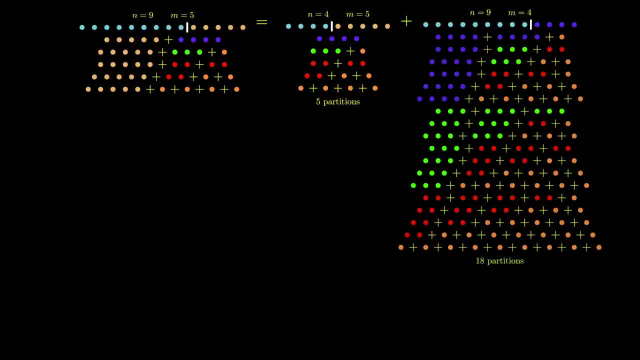 parts up to m minus one. Here are the partitions for the n is equal to four and m equals five case. By adding m to each of these partitions, we generate the corresponding subset of partitions for the n equals nine and m equals five case. And combining this with the 18 partitions from: 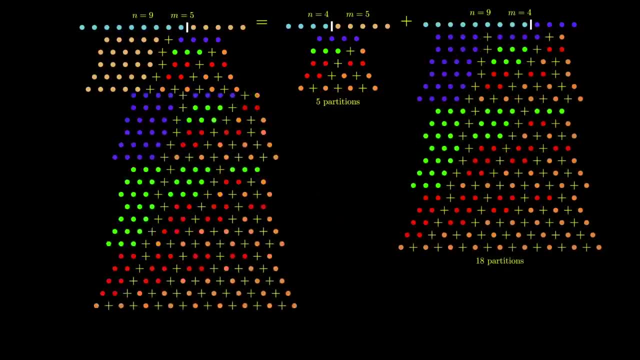 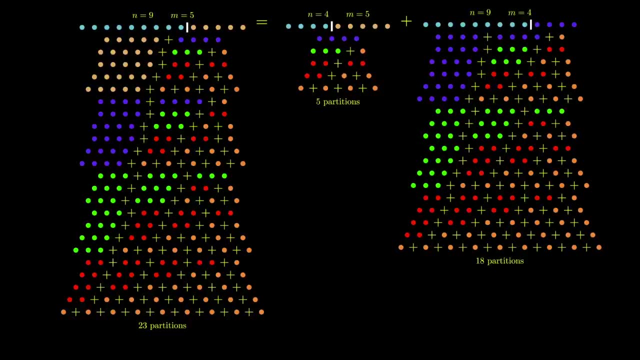 the n equals nine and m equals four case, we end up with 23 total partitions for the n equals nine and m equals five case, And you can take the time to verify this if you wish, but these do actually end up being all the partitions for n equals nine and m equals five case. Okay, let's now generalize. 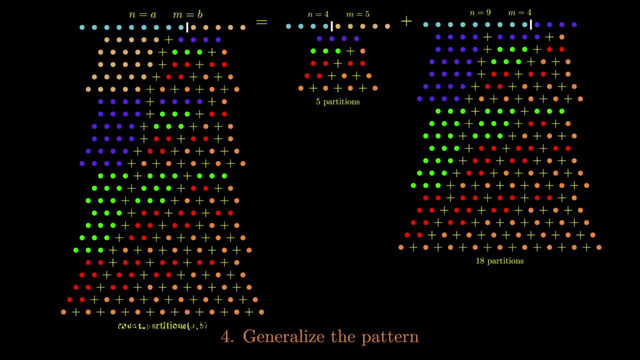 this pattern If we want to solve the count partitions problem called on a and b, it will end up being the sum of the count partitions called on a minus b and b, and then count partitions called on a and b minus one. This is the key recursive relation that will solve this problem. 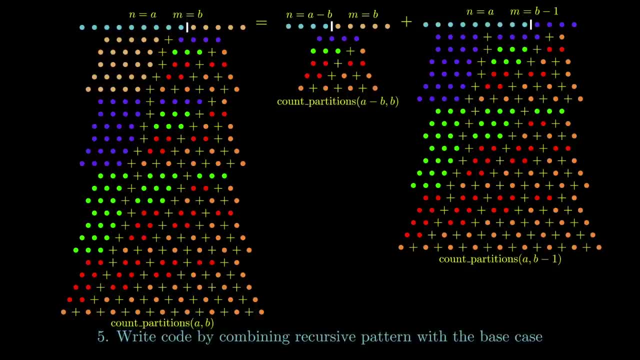 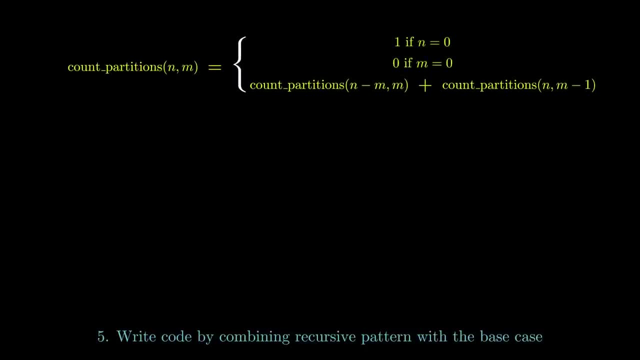 Let's now execute the final step and put together our recursive relation with the base case. One interesting wrinkle that we will have to take account of is that one of our recursive calls provides an argument that is n minus m. Some of you may have noticed. 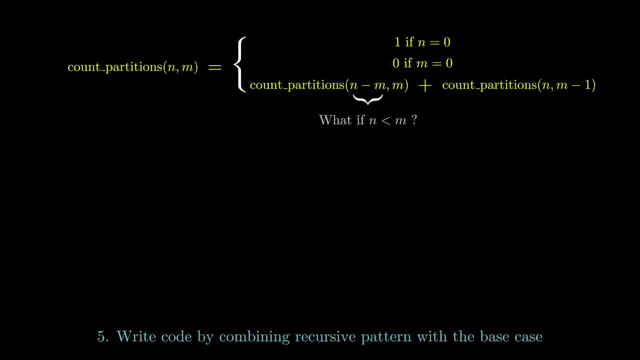 that it's perfectly valid to have cases where n is actually less than m, which then means that the new call will have a negative argument. To account for this, we have to include this corner case in one of our base cases. If the n value provided is negative, we will have zero partitions. This: 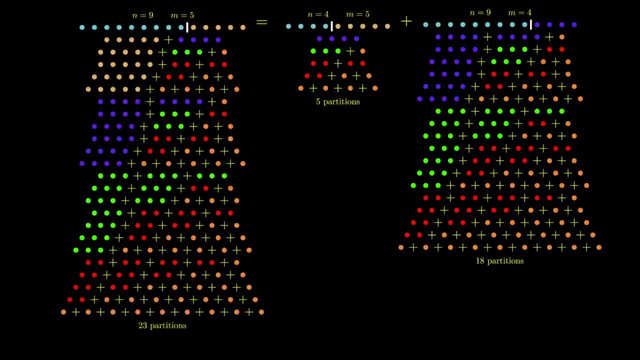 total partitions for the n is equal to 9 and m is equal to 5 case, And you can take the time to verify this if you wish, but these do actually end up being all. the partitions for n is equal to 9 and m is equal to 5 case. Okay, let's now generalize this pattern If we want to solve the count. 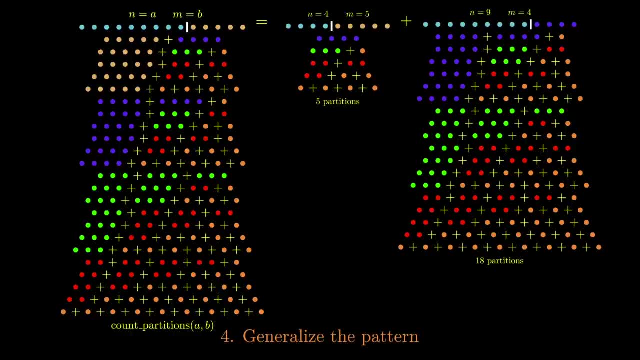 partitions problem. called on a and b, it will end up being the sum of the count partitions called on a minus b and b, and then count partitions called on a and b minus 1.. This is the key recursive relation that will solve this problem. Let's now execute the final solution. 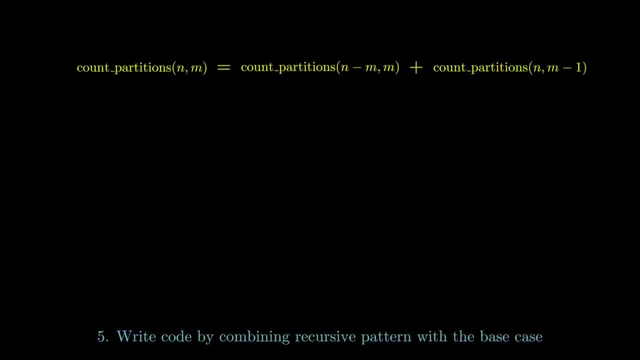 step and put together our recursive relation with the base case. One interesting wrinkle that we will have to take account of is that one of our recursive calls provides an argument that is n minus m. Some of you may have noticed that it's perfectly valid to have cases where n is actually. 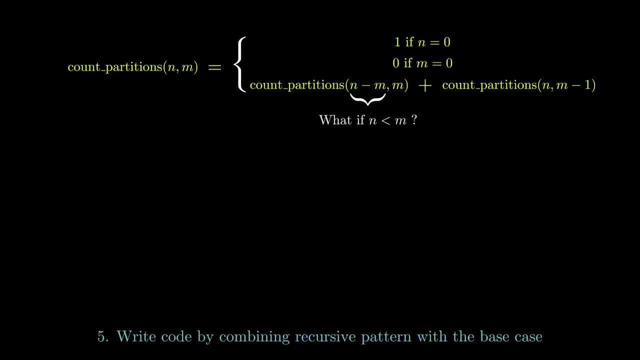 less than m, which then means that the new call will have a negative argument To account for this. we have to include this corner case in one of our base cases. If the n value provided is negative, we will have zero partitions. This problem is a good example of how you might have to modify some. 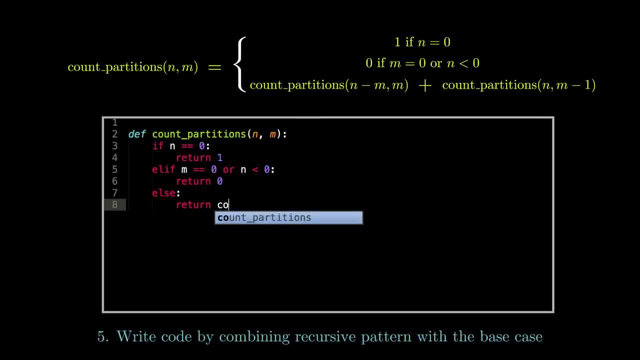 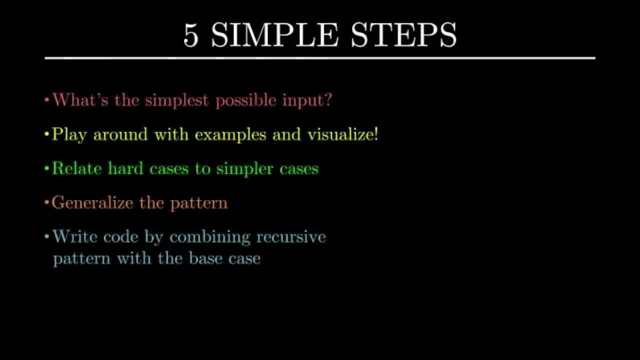 of your base cases after finding a general recursive pattern. The cool thing about recursion is that for such a tricky problem, our final solution actually ends up being only six lines of code. So to recap what we did in this video, we went over five key steps to solve any recursive problem. 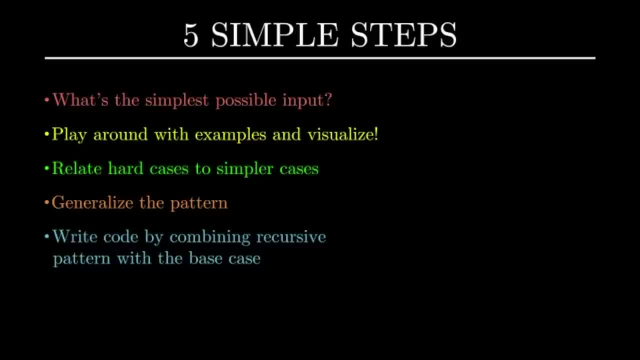 and then went about applying these steps to three problems of various difficulties. You learned the importance of starting simple and asking yourself what the simplest possible case is. You found it helpful to work through some examples to get a sense for what the recursive problem was asking. You also went about relating hard examples to easy examples to find a 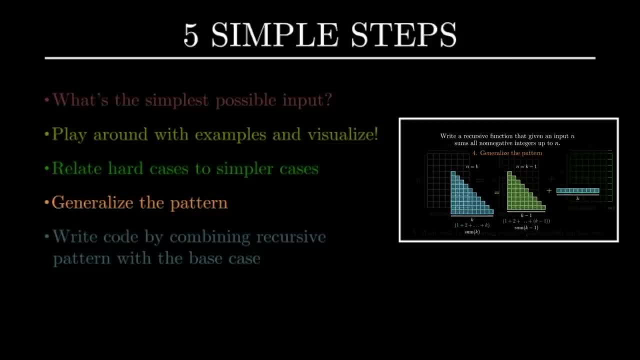 generalizable recursive pattern And then, with this pattern in hand, you went about writing the code. As with anything you learn, you're going to have to spend some time to really contemplate and work through recursive problems to really begin to master solving them. 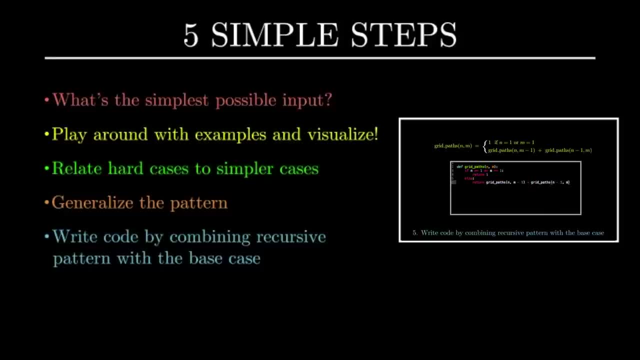 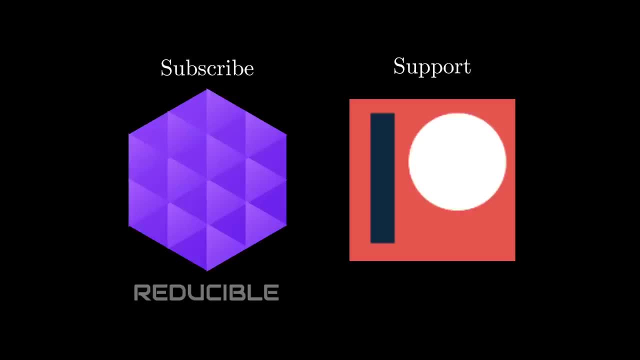 This video is all about giving you a mental framework to do that, and I hope it was helpful in that sense. Thanks for watching and, as always, I'd appreciate it if you liked the video, if you enjoyed it. If you want to see more content like this, be sure to hit the subscribe button and if 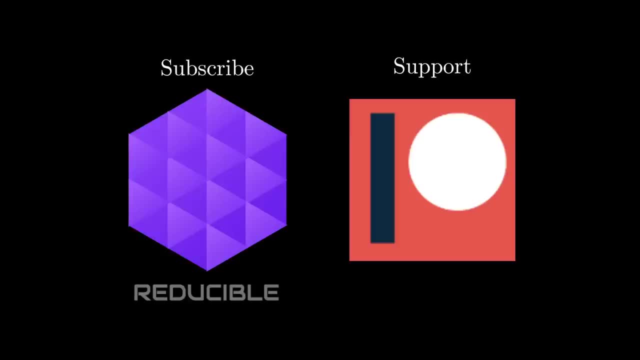 you want to more directly support this channel, be sure to check out the Patreon page linked in the description below. See you in the next video.